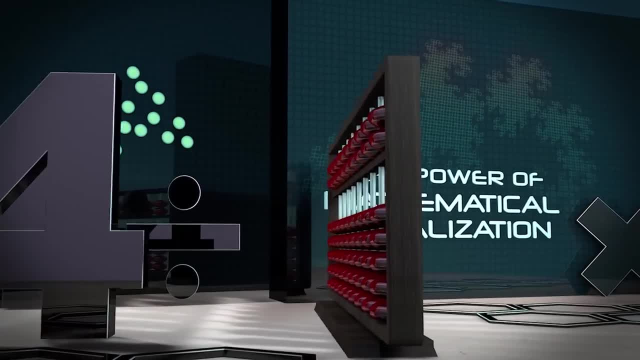 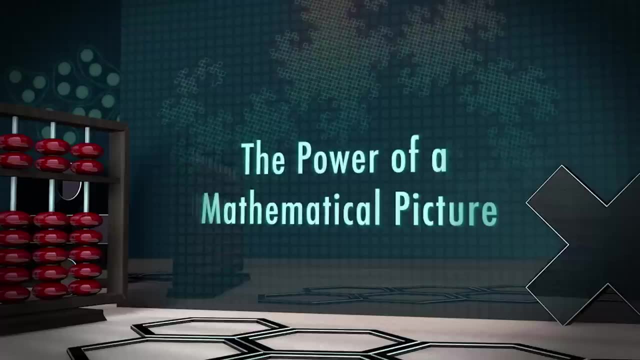 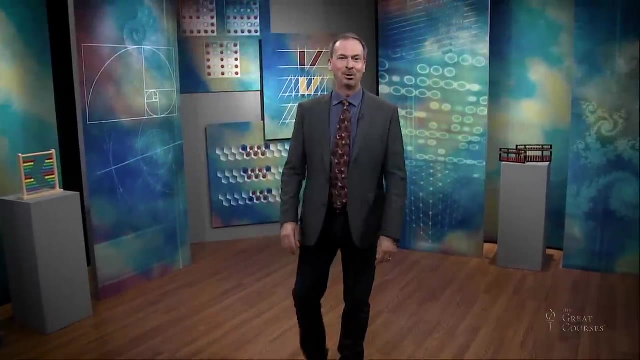 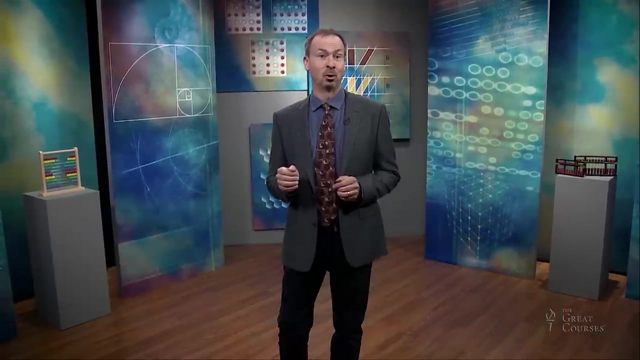 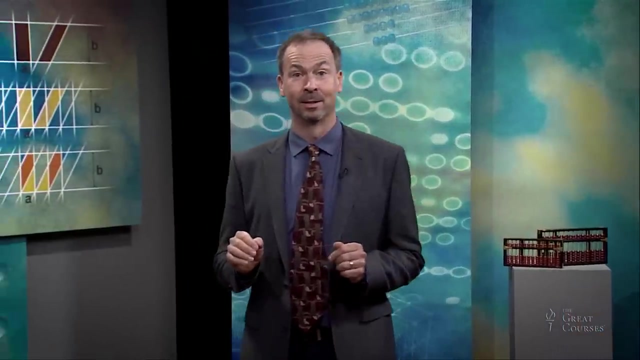 G'day. I'm James Tanton and I'm absolutely thrilled to be with you for this series and to share with you what I believe to be a key component to joyful mathematics success: the art of being visual. They say a picture can speak a thousand words. Well, in mathematics. 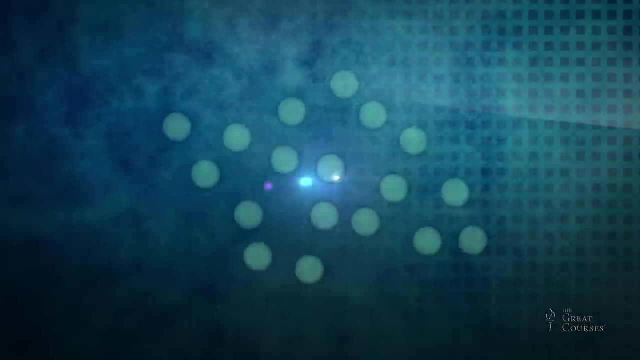 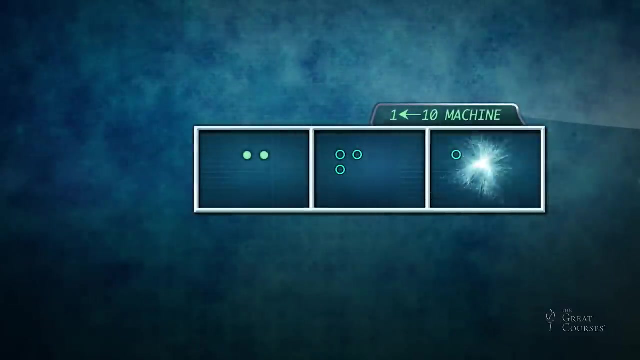 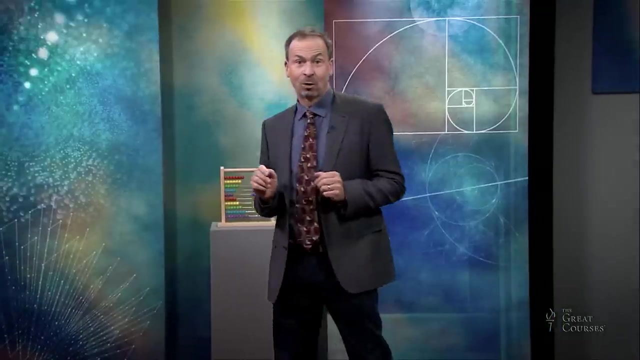 a picture can spawn a thousand ideas. A picture can provide deep understanding. A picture can prompt that aha moment to cause an idea or process to suddenly make sense. A picture can lead to finally understanding a tricky piece of mathematics, And that's what this course is about. 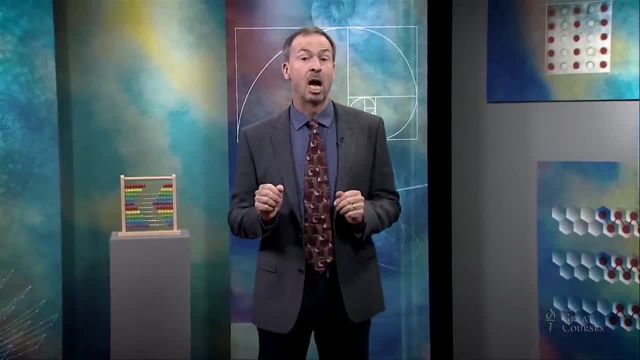 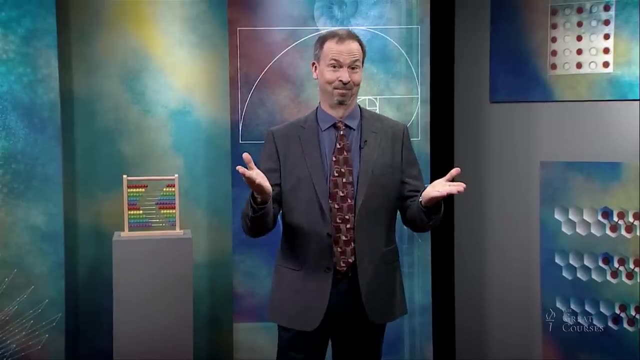 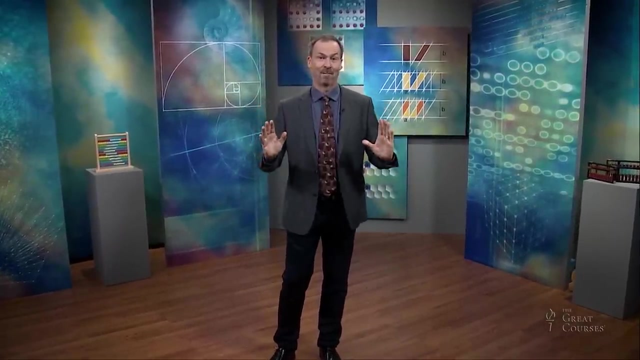 I want to share an alternative way in to the subject, a way to think about topics and see- truly see- what they are really about and how to make them work for you. Now, the ideas can be elementary or they could be advanced, It really does not matter. All mathematics, all levels of 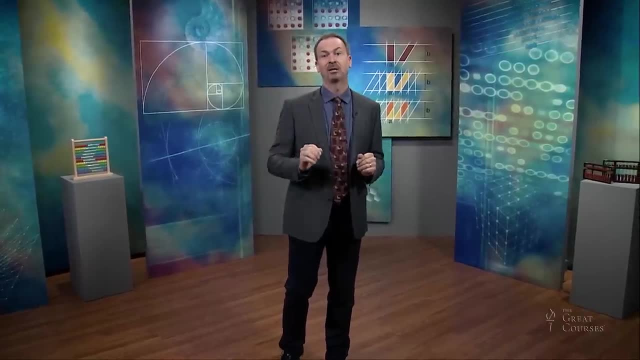 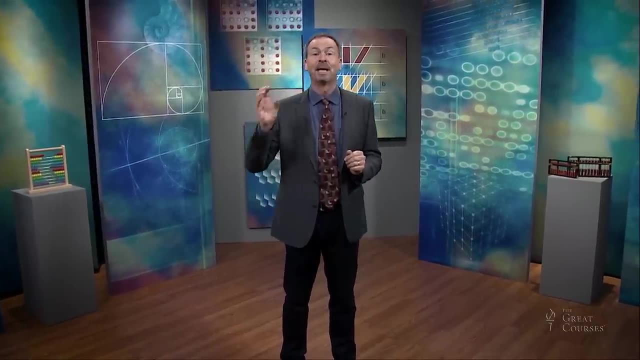 mathematics, if thought about with intentionality, naturally lead to beautiful, clever and powerful ideas. Whether a simple study of counting or study of tricky probability theory, every piece of mathematics serves as a portal for further thought and wonder. In this course, I will show you how. 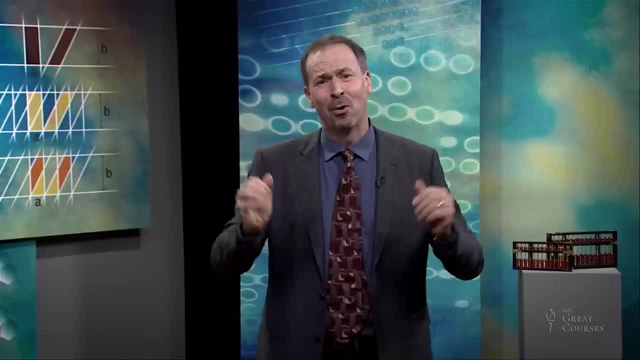 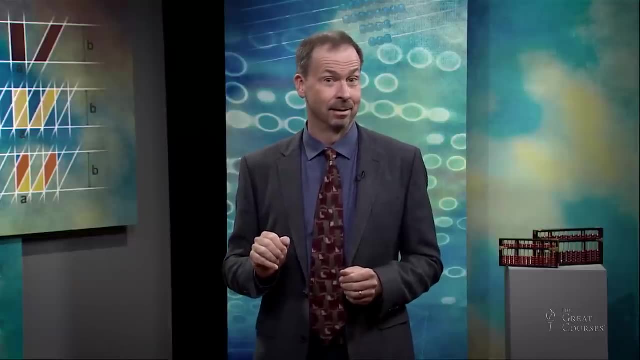 The story of visual thinking in mathematics is a very personal one for me. I grew up in Australia and my mathematical training in my K through 12 days wasn't particularly enlightened. This was back in the 70s. We were taught algorithms, arithmetic algorithms in primary school, algebra algorithms. 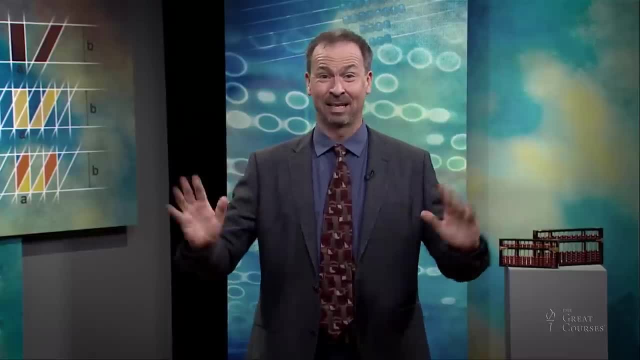 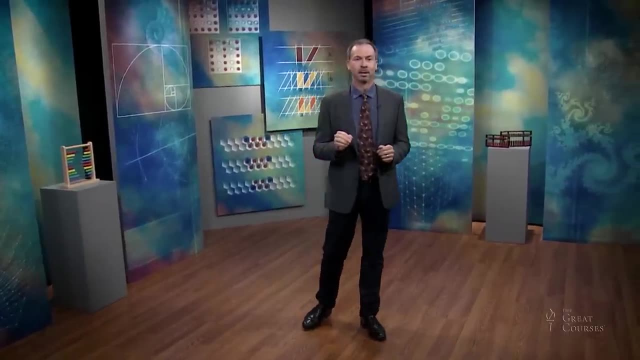 in high school and so on, And I got the message loud and clear that my job was just to do and not to question. But I want to know why these algorithms worked. I want to know why negative times negative is so important. I want to know why negative times negative is so important. I want to 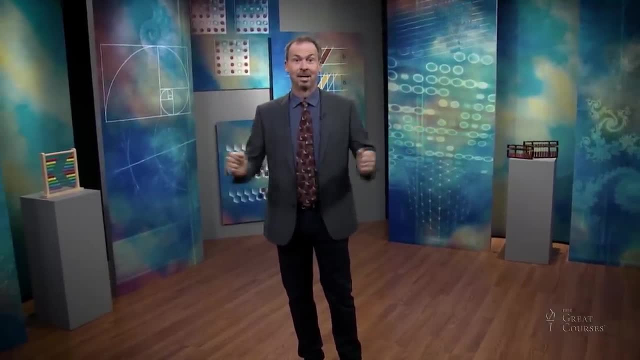 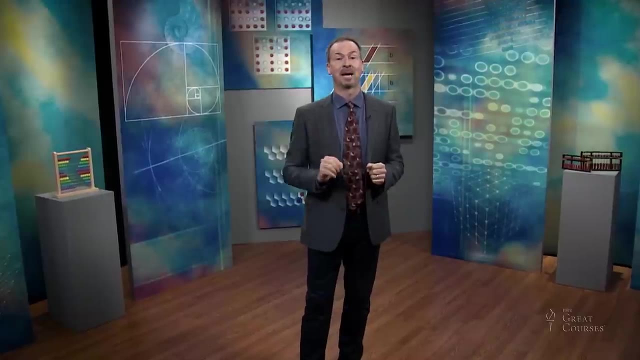 know why positive is positive other than just being told it is. I want to know why all the patterns in Pascal's triangle work the way they do, and so on. But I learned early on I was not to ask questions, My job was just to perform, And perhaps your experience was similar to mine, Perhaps you 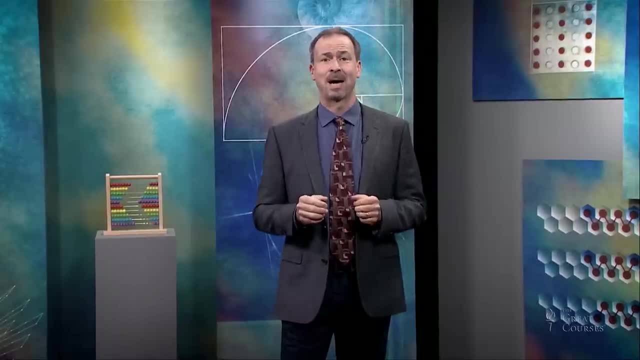 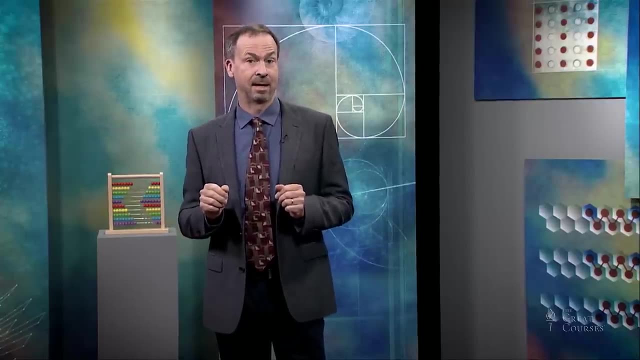 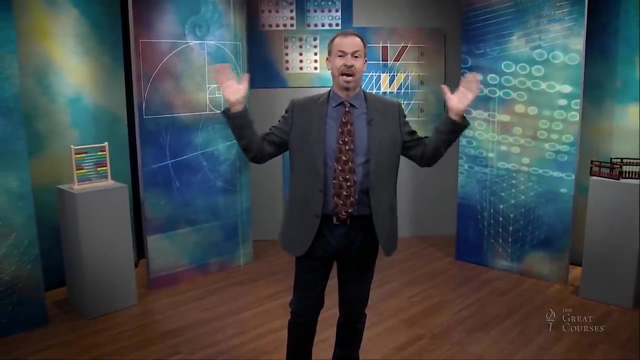 too, want to know why. We can all thank heavens that mathematics education is much more enlightened today, But there was something in me that compelled me to make sense of things nonetheless. I had pictures. The very early grades in my schooling were all about pictures. We drew shapes and counted dots. 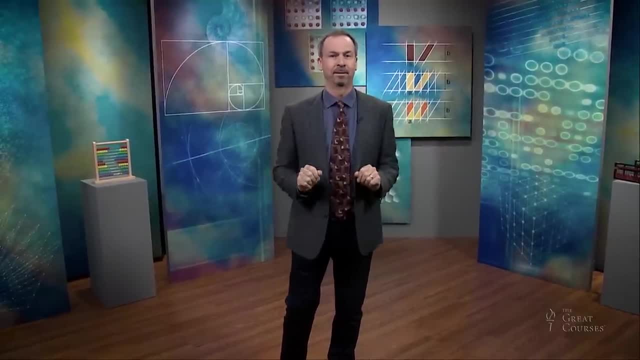 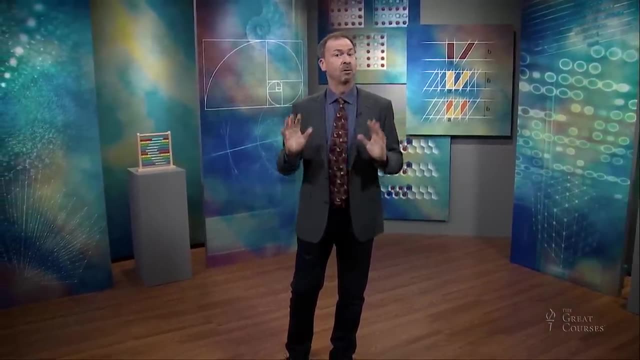 We did all sorts of wonderful visual things. All good stuff. But then matters changed from grade four onwards. for me, Working with pictures was no longer considered valid, No longer valid mathematics. Their status changed to that of simplistic tool suitable only for the very young. 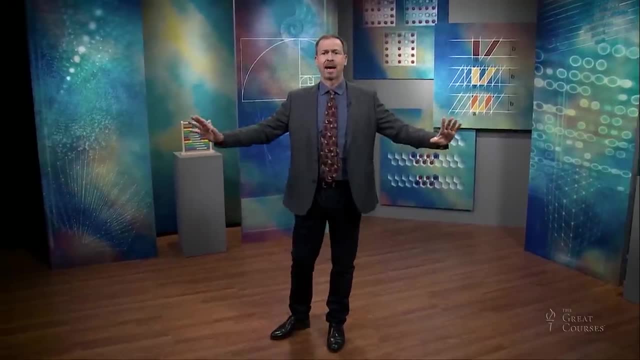 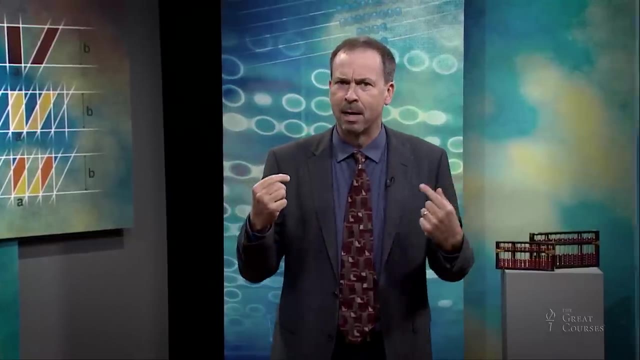 Our job was now to think analytically through equations and numbers on the page, and not visually. But something in me kept holding me back. I was not to think analytically, I was to think of my own thoughts. I thought of visual thinking. nonetheless, Privately in my mind, I knew for me. 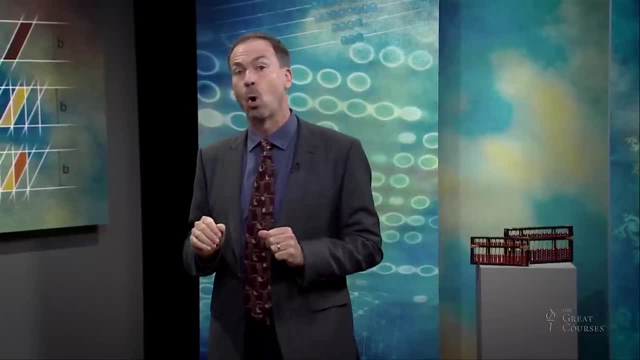 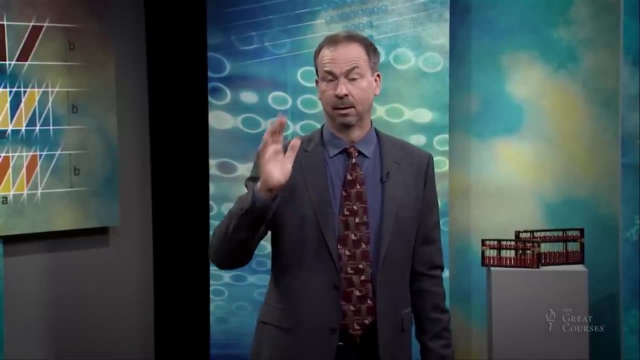 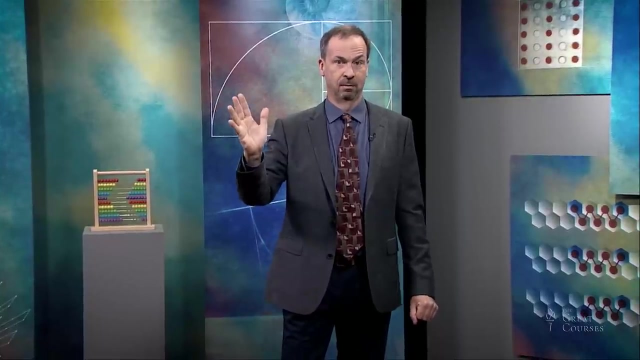 pictures were a key to understanding, Even for the mathematics given only in equations and words. So let me show you what I mean. Here are some examples from basic arithmetic. Okay, Division: I remember in my early grades circling groups of dots and pictures to make sense of division. For 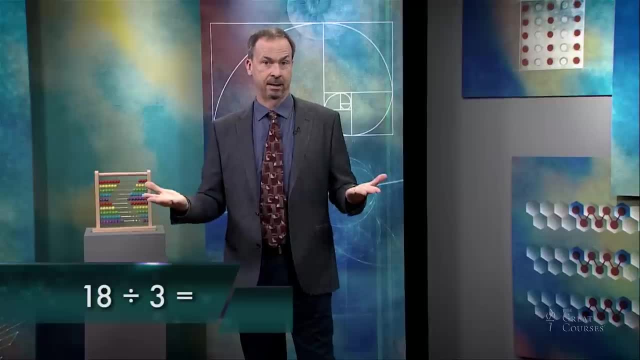 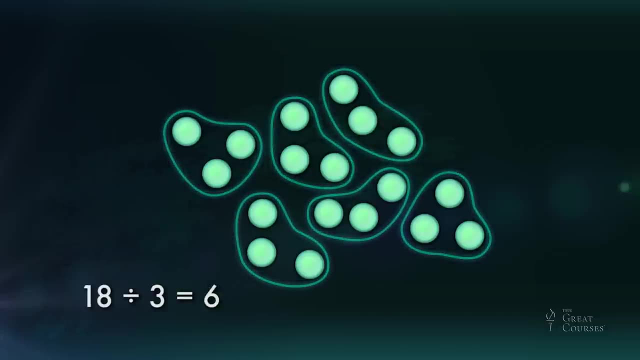 example, the division problem, 18 divided by 3, is asking: how many groups of three can you find in a picture of a of 18 dots? Well, there are six of them. Super 18 divided by 3 is 6.. And then I remember years. 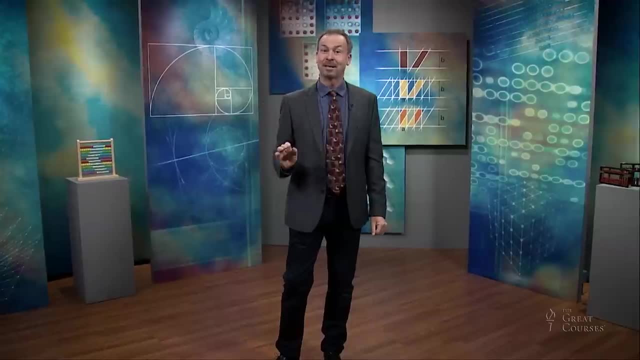 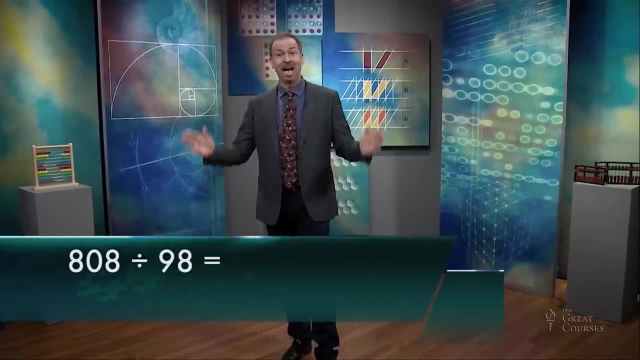 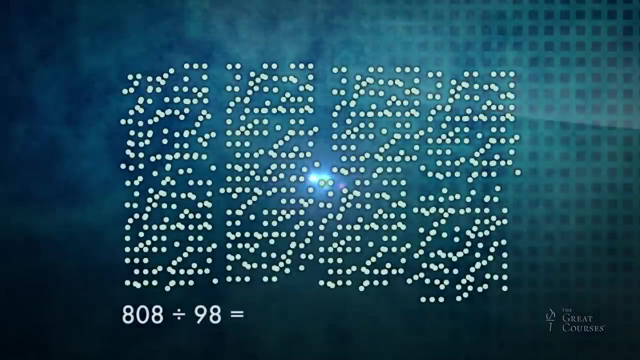 later having the realization that I can push this visual picture further and make sense of some complicated division problems. For example, 808 divided by 98. I could just see it had to be 8, with a remainder of 24.. Here's what my brain imagined. We're looking for groups of 100. 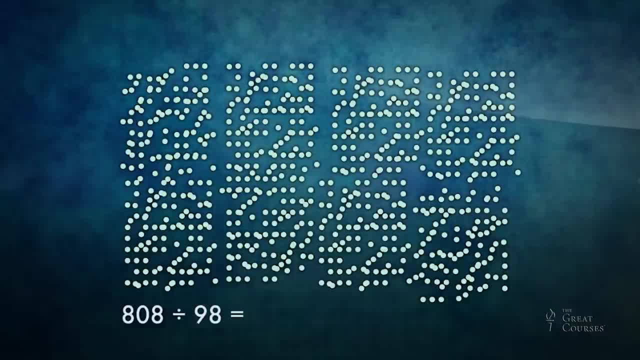 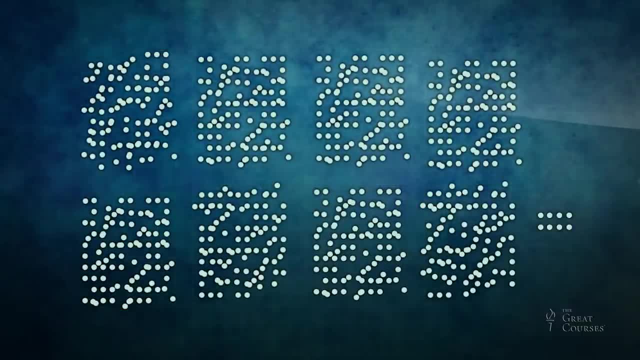 rather than 98. The number 98 is just too hard for me to fathom, So look for groups of 100 instead, And we can see there'll be 8 of these groups with 8 dots left over. Ah, but each group. 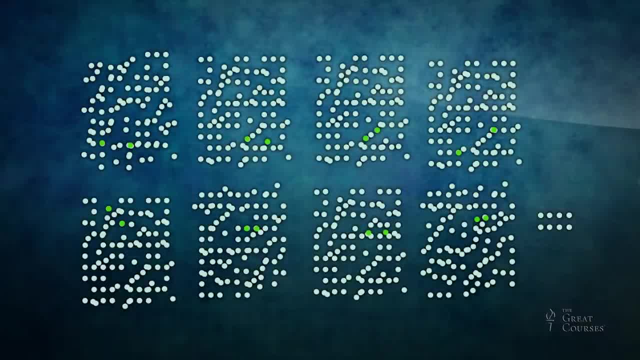 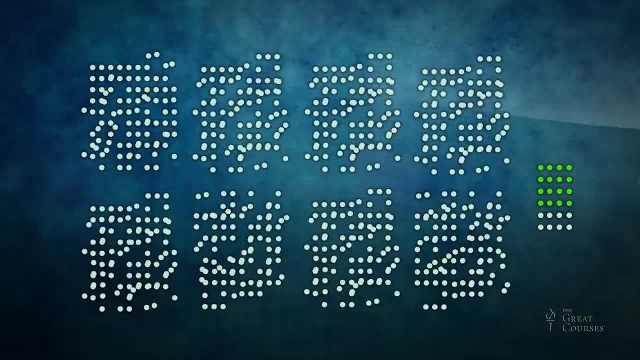 of 100 is itself off by 2 dots. We wanted groups of 98 after all, So we have an extra 16 dots floating around as well. So that makes for 8 groups of 98 and a remainder of 16 and 8. That 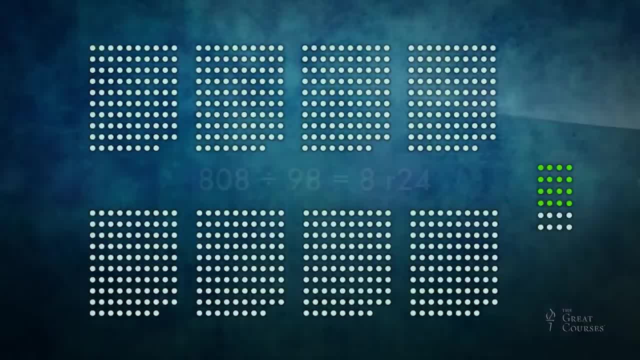 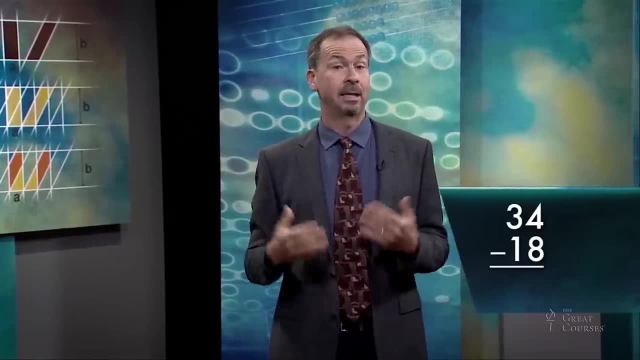 is a remainder of 24 dots 808 divided by 98. Is 8 with a remainder of 24.. Just like I said, I could see it Subtraction. When asked to do 34, take away 18,, I could certainly do the standard algorithm and get the answer 16.. But can't we? 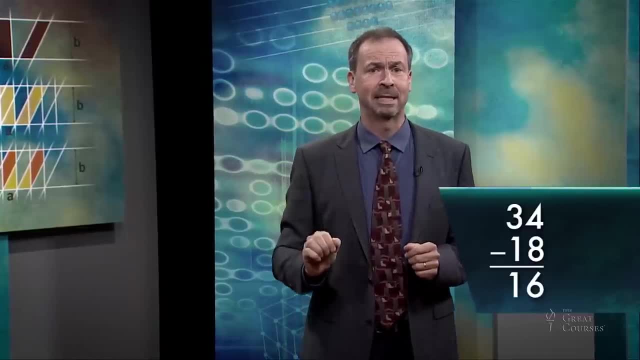 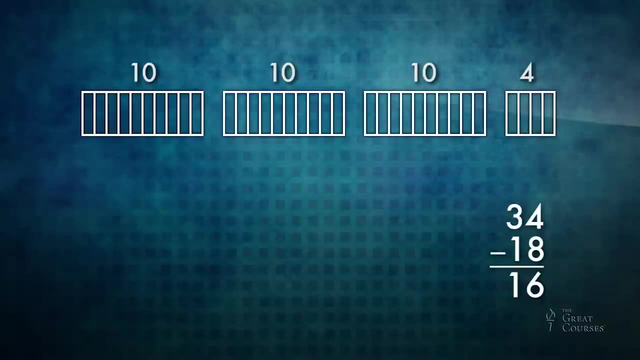 just see in our minds, the answer just has to be 2 plus 10 plus 4, which is 16?. Line up a row of 34. the two rows differ by 2 and 10 and 4 blocks. The difference is 16.. In the same way, 1,012. 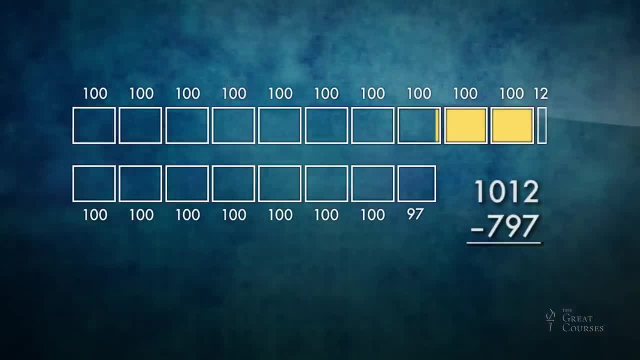 take away 797, just has to be 3 and 212.. That's 215.. Can you see that 797 to 800 is 3.. 800 to 1,000 is another 200. And the extra 12 gets me to 215 in total. Actually, this flexibility. 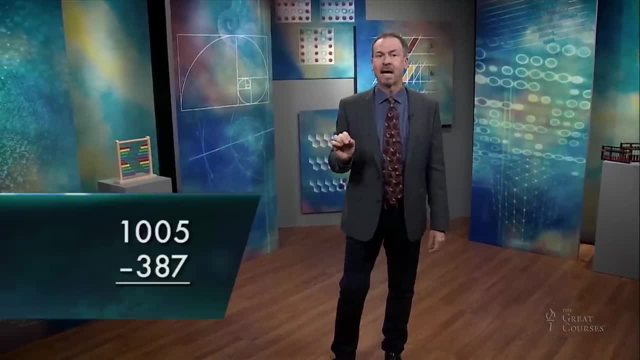 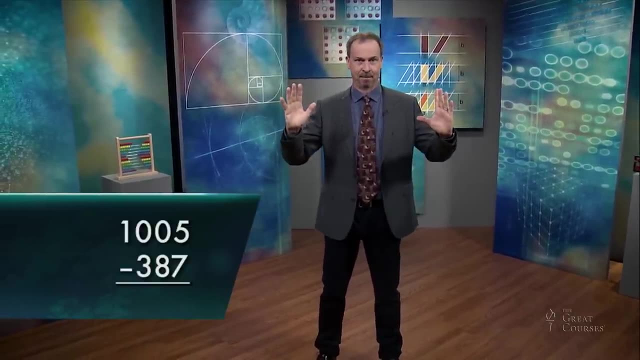 of thought helps subtraction in general. For example, look at 1,005, take away 387.. All right, In the classic way of doing this, we have a lot of borrowing to do here, That is we have to do: 5. take away. 7 requires a borrow 0. take away 8 requires a borrow 0. take away 3, yet another. 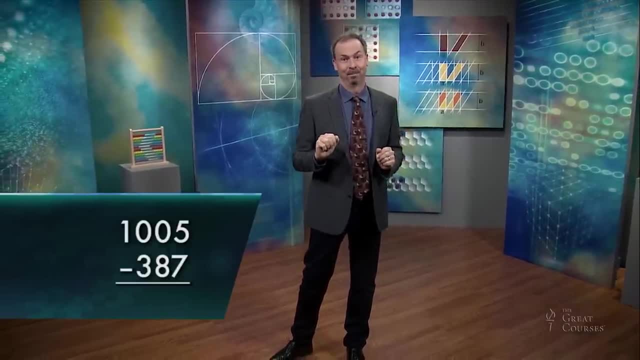 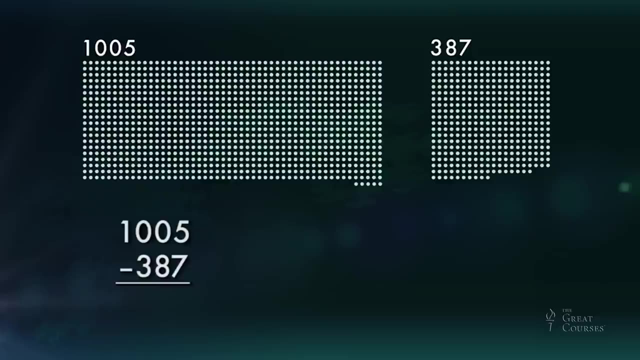 borrow. But we can make this work simpler. So here we're looking for the difference between 1,005 dots and 387 dots. So let's make the 1,005 friendlier and turn it into 1,000.. Just remove 5 from each pile and let's just compute the difference. 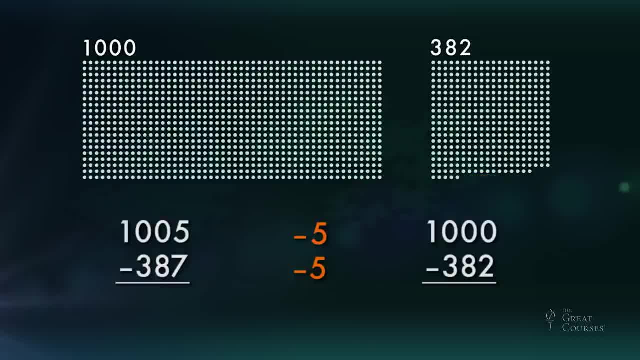 between 1,000 and 382. instead. Now I can see in my head the answer has to be 8 and 10 and 600.. 8 to get up to 390, 10 to get to 400, 600 to get up to 1,000.. Total of 618. Ah. 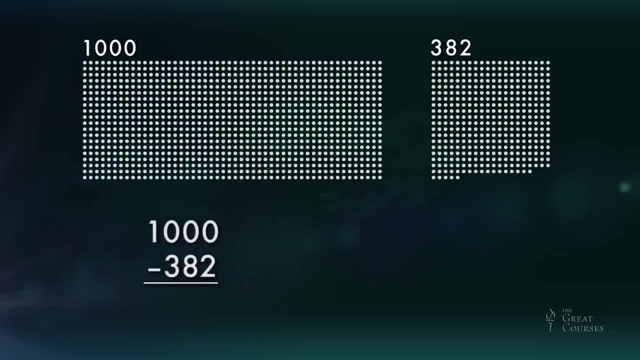 but if I don't trust my head and still want to do the traditional algorithm, then I suggest remove one more dot from each pile and make the problem 999, take away 387.. Now I can do the algorithm without any borrowers whatsoever. 9 take away 1, fine, 9 take away. 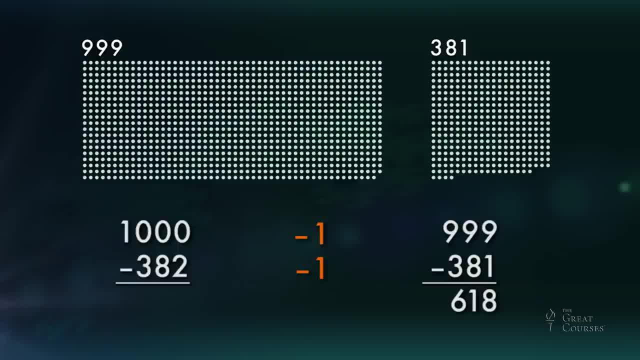 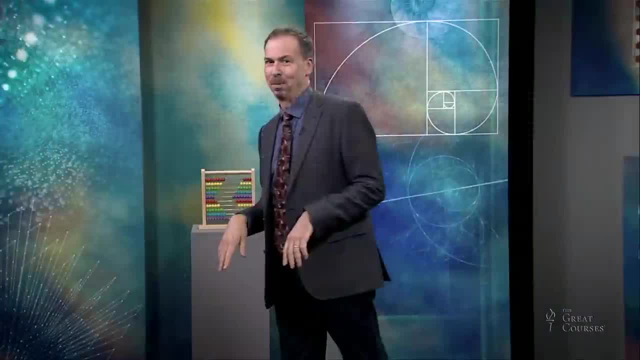 8, no problem. 9: take away 3, piece of cake. I've made the problem so much easier to do, even if someone insists that I use the algorithm Fine Multiplication. Isn't multiplication really a geometry problem? Isn't 24 times 13,, say? 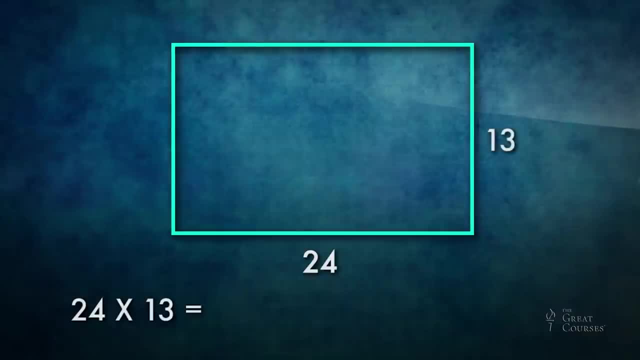 just asking for the area of a rectangle that's 24 units wide and 13 units high. Then why not just chop the rectangle to pieces that are much more manageable? For example, think of 24 as 20 and 4 and 13 as 10 and 3. Then I can see that 24 times 13. 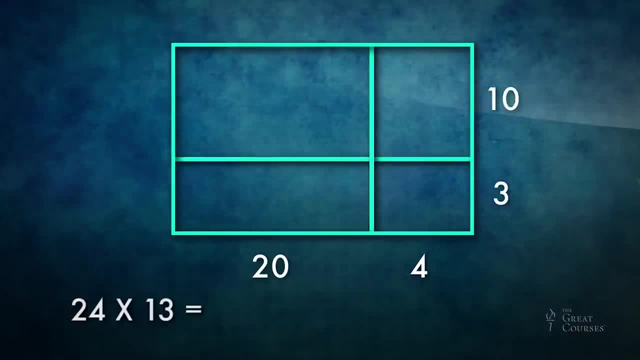 must be the areas of the individual pieces added together. There's 200, there's 40, there's a 60 and a 12. That's 312.. This type of visual thinking is only the beginning, the very beginning. These are pictures of the whole picture. They're not just pictures of the. 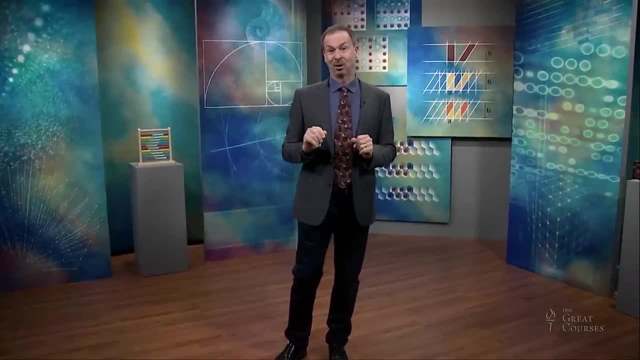 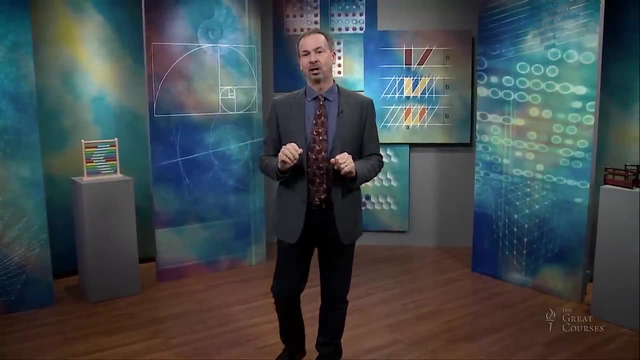 whole picture. They're pictures to go with grade school arithmetic. But we can mull on and tweak these pictures further and we'll see how they can provide gateways to so much more. For example, our picture of multiplication can be used to make perfect sense of why negative times negative is. 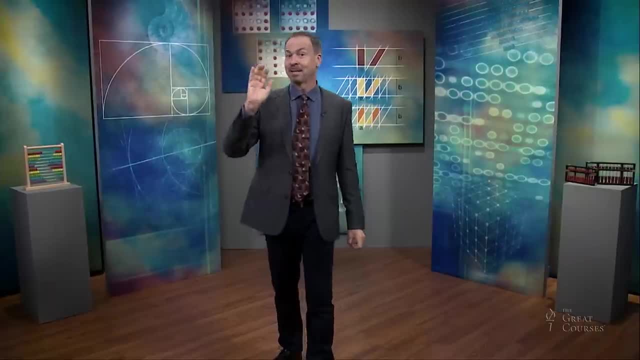 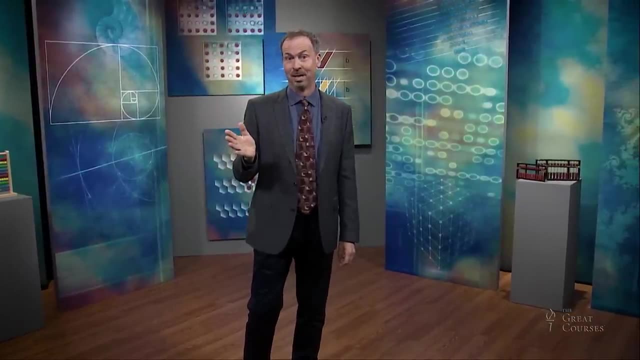 positive- And we'll do that a bit later in the course- And we can make sense of expanding brackets in algebra class, which then takes us to advanced ideas such as connecting Pascal's triangle to algebra, and which will then take us to results in statistics and so on. Each picture: 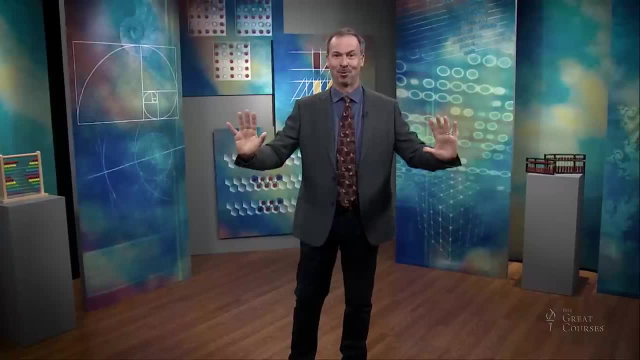 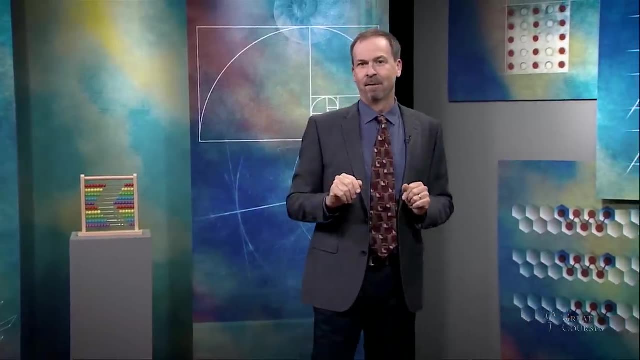 we draw, like I said, is a picture of the whole picture, And we can make sense of expanding brackets to so much more. We'll see this over and over again throughout this course. For some reason, visual thinking was in my bones from the get-go, And I actually think I know why. 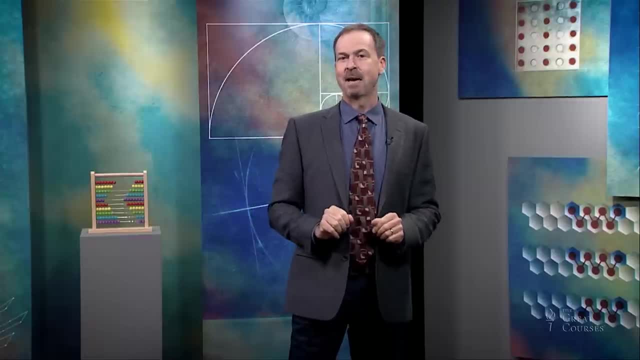 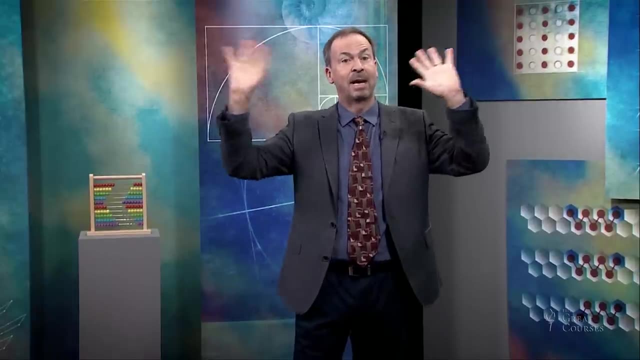 Back in Australia back in those days in the 60s and 70s, my family owned an old Victorian house. It was my childhood home And each room of the house had a pressed tin ceiling And each had some decorative design on it and printed on it in some way, And this included my bedroom. 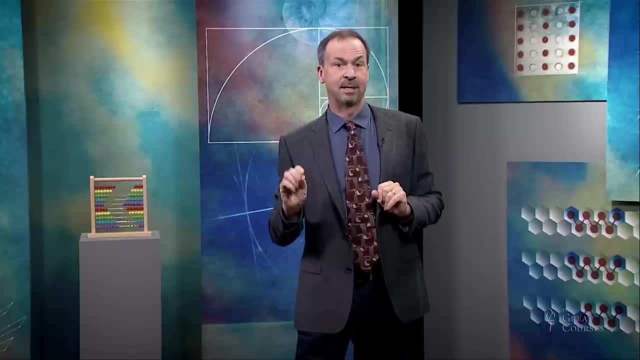 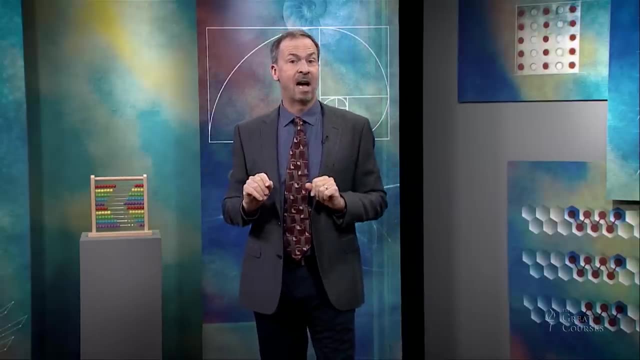 and I spent each and every night of my childhood falling asleep staring at the design on my bedroom ceiling. And the design I had on my room was particularly striking. It was just a five-by-five grid of squares. Now the edges were vines and the corners were little flowers, But in the end 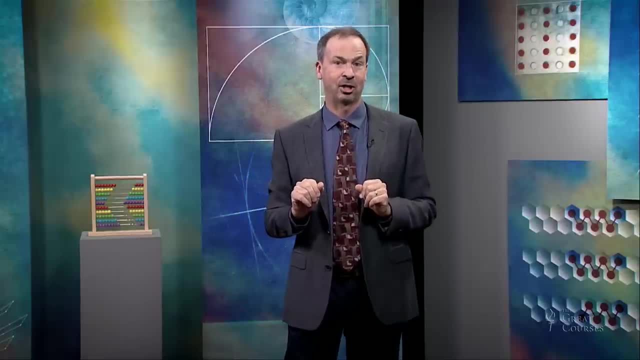 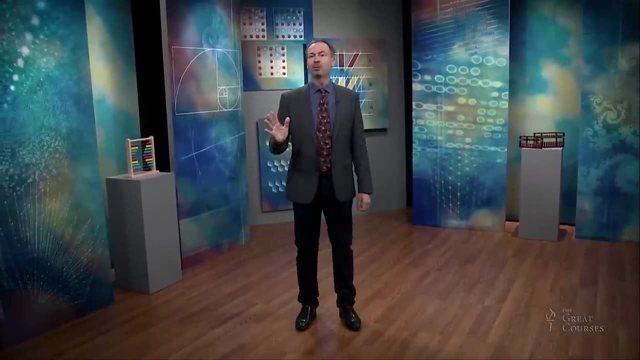 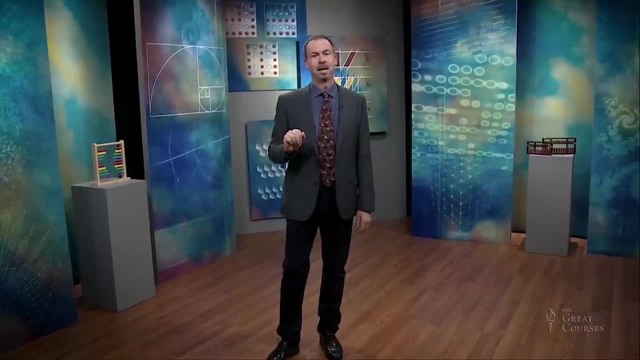 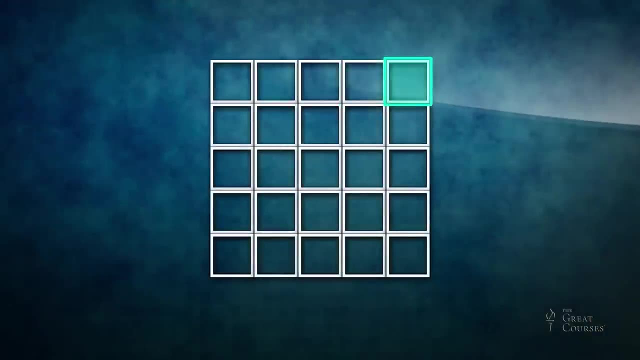 And mind games based on that grid of squares, And I remember my very first mathematic surprise coming from counting on that grid. It's this one: Clearly, there are 25 little one-by-one squares in the grid, But we can count two-by-two squares as well, And there are lots of. 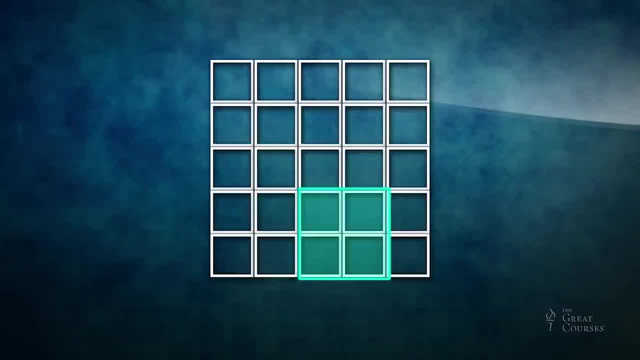 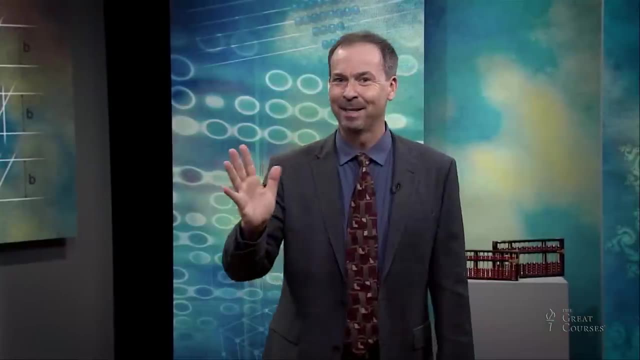 those, I end up counting 16 in total. And then I counted the three-by-three squares, And it turns out to be nine of those, And the four-by-four squares- There are four of those- And finally there is one big five-by-five square. Now look at these: counts Twenty-five. 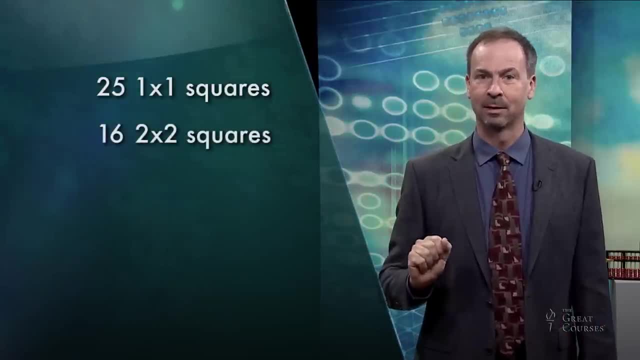 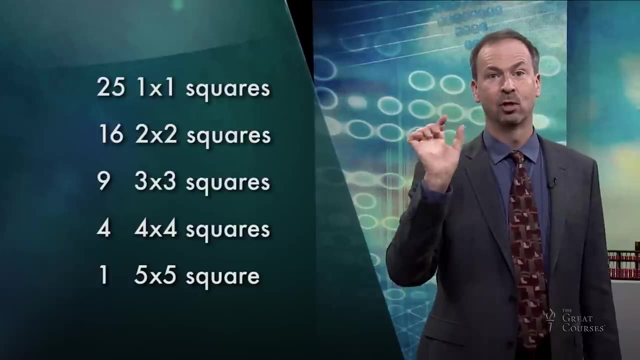 one-by-one squares, Sixteen two-by-two squares, Nine three-by-three squares, Four four-by-four squares And one five-by-five square. Each count 25,, 16,, 9,, 4, 1.. Each count of squares is itself. 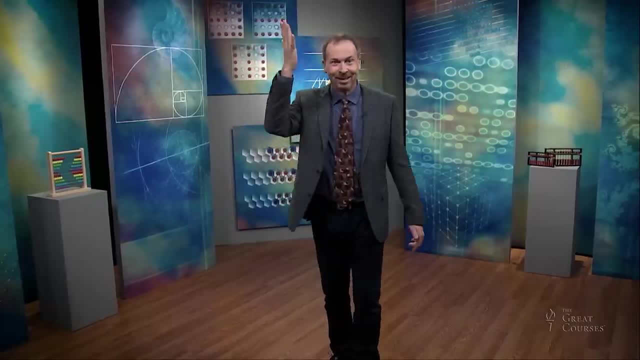 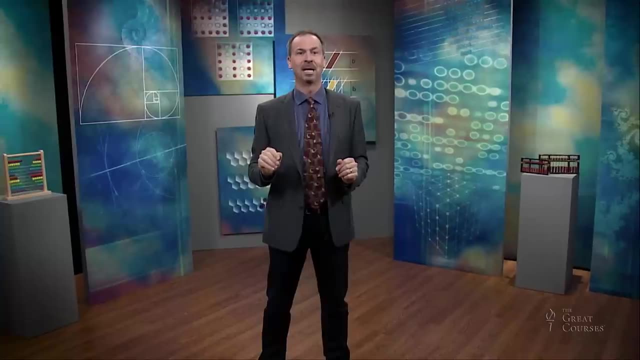 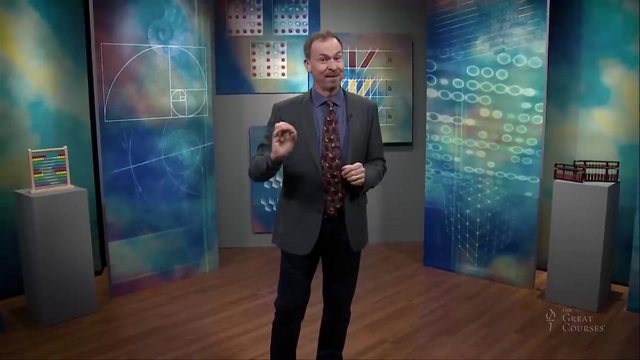 a square number And I found this striking. I found it surprising And I want to know the why, How I might change tautology. Counting squares on a square grid gives square-number answers And it took me a long while to figure out how to explain what was going on. My epiphany was to focus. 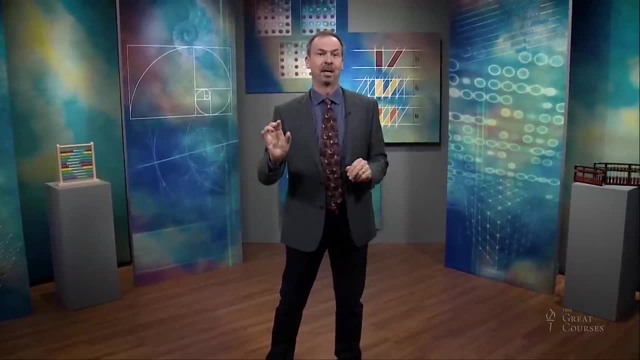 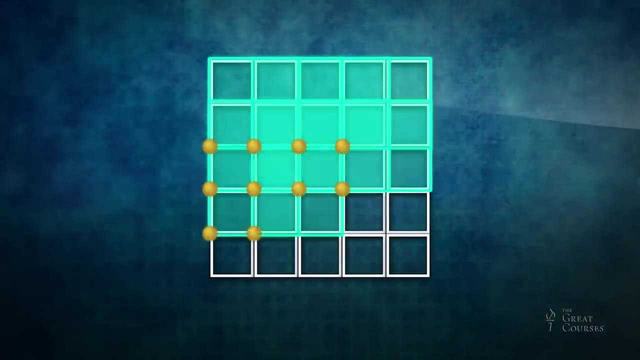 on the lower left corners of squares. I was counting, For example, of the two-by-two squares. there are some possible lower left corners. now let me draw all the possible lower left Corners. And now I see there is a UP list of the FOUR-by-icing squares. 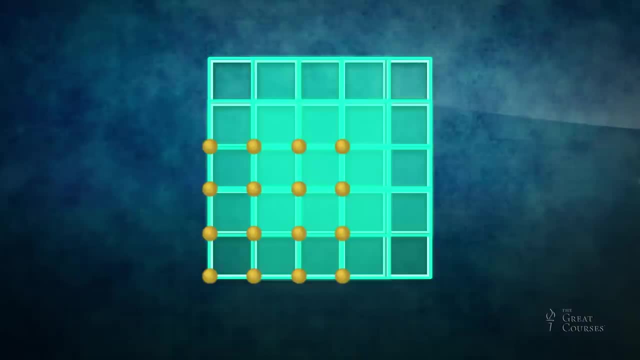 are the possible lower left corners. Now let me draw all the possible lower left corners. And now I see that there is a square array of the them. Assad Faihina supplements these patterns this time 4 times 4 of them, in fact, that's 16.. 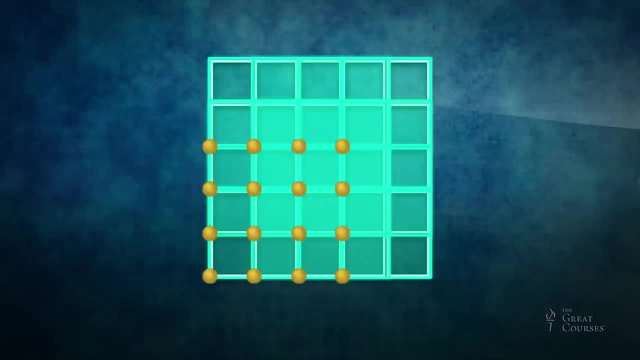 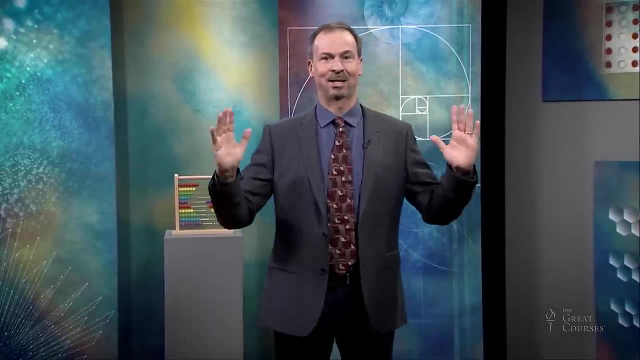 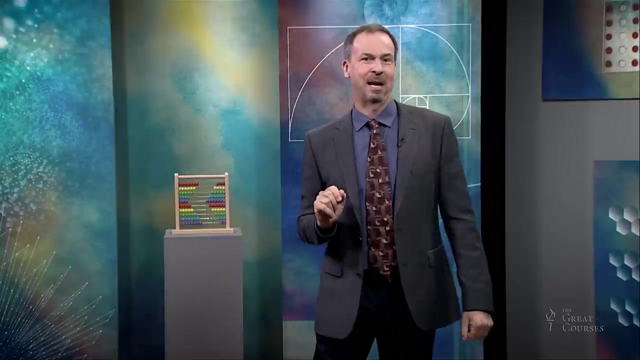 Thus there are 16 2x2 squares. This image just made it clear to me why the count of squares is always sure to be a square number. Very exciting, But there was one puzzle I made up for myself on this grid that I truly believe made me a mathematician. 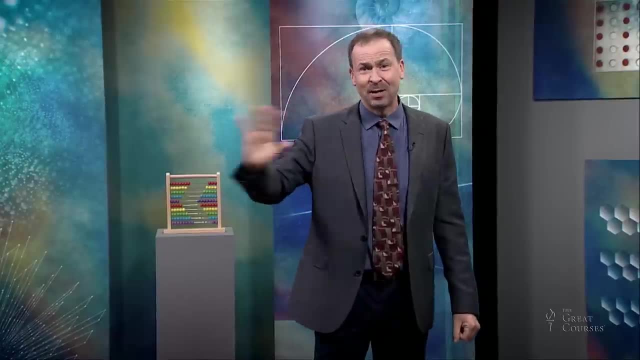 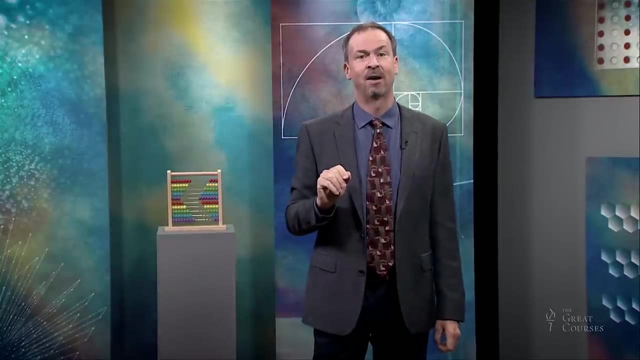 It wasn't until years after my schooling, in fact doing university mathematics, that it came to me that I realise now I was doing visual thinking and was actually doing mathematics on that 5x5 grid of squares. I realised then that this bedroom ceiling. 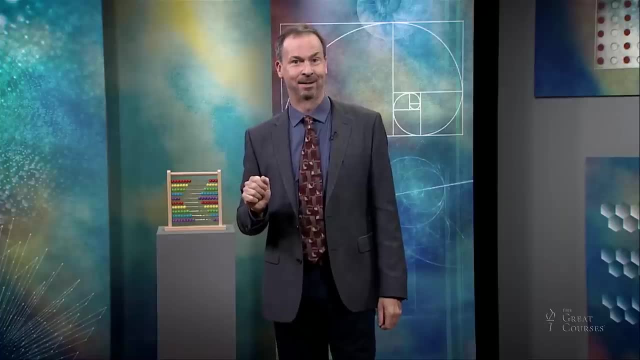 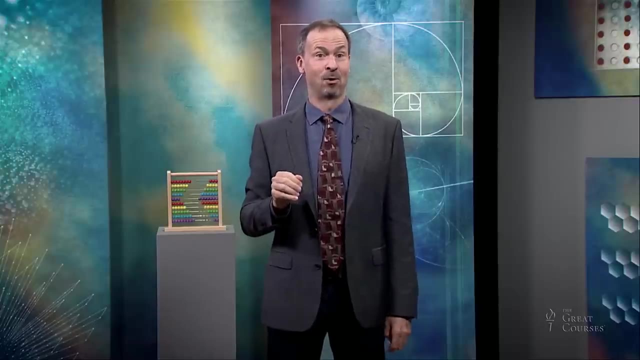 was actually my portal to true mathematics, And I would encourage you to look for a similar opportunity. Perhaps you, too, have ceiling tiles or a wallpaper pattern or a parquet floor or a tiled floor, something you look at every day, And once you start looking for these patterns, 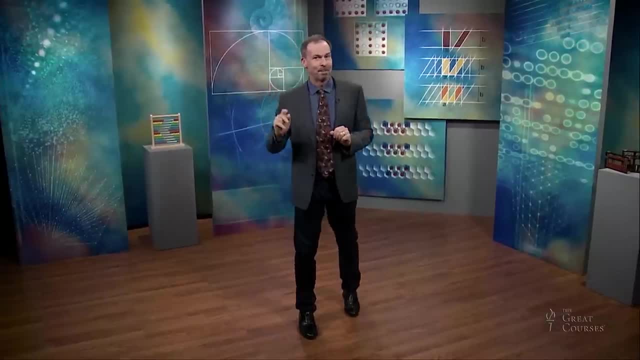 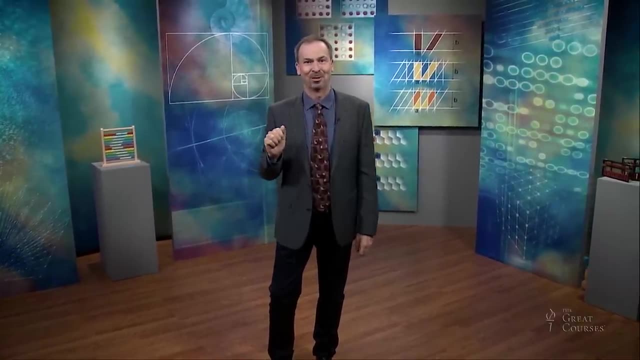 you'll be amazed at how many you'll find. So to explain the puzzle- the one that made me a mathematician- I'm going to work on an actual grid of squares with you. So let's head on over and do a demonstration. 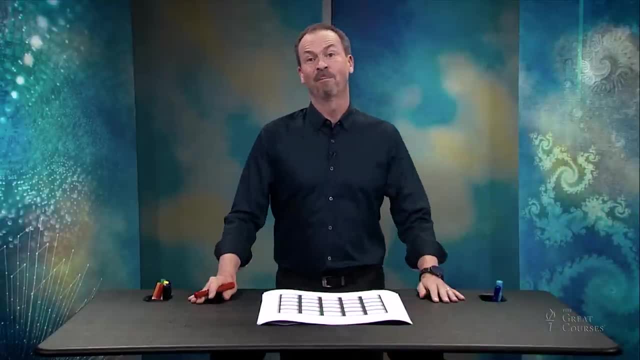 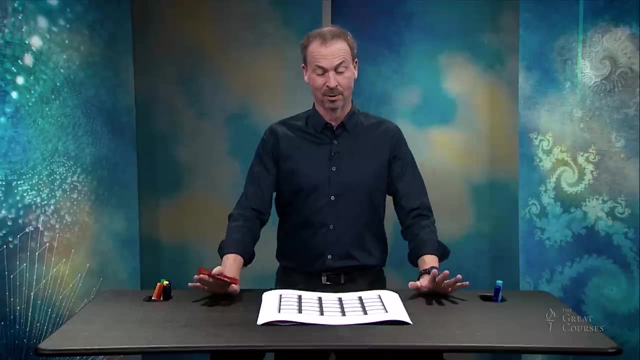 OK, here it is, my bedroom ceiling: a 5x5 grid of squares. And here's the puzzle I invented for myself. that, I truly believe, made me a mathematician. It goes as follows. So I chose a starting spot. 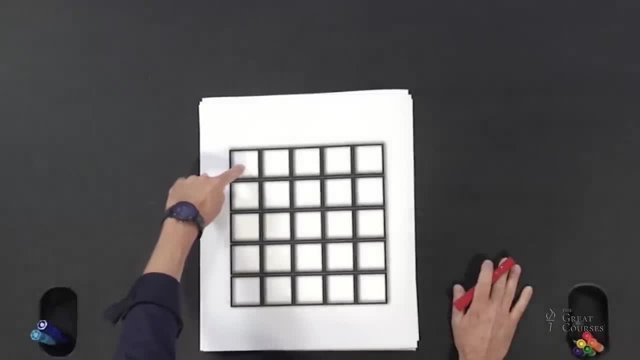 So let's say I chose the top left corner And the game I played for myself was: can I walk a path that visits each and every cell exactly once, just moving horizontally and vertically? And, for example, I can actually do it. 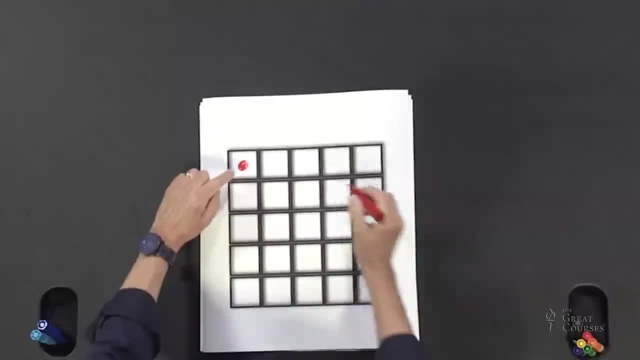 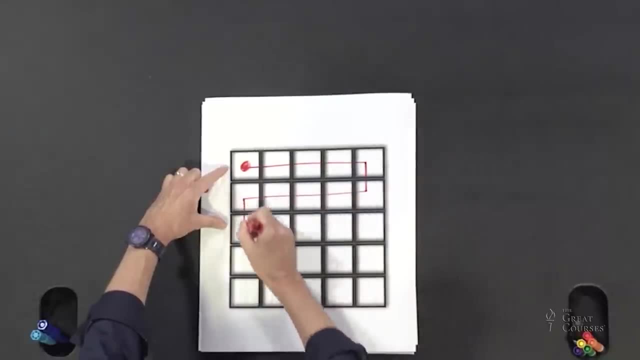 This one does work. So I'll start here, I'll mark my starting spot And maybe I'll do a whole bunch of horizontal steps first, Maybe, then one down step vertical, Then maybe another bunch of horizontal steps, And then I can keep going this way. 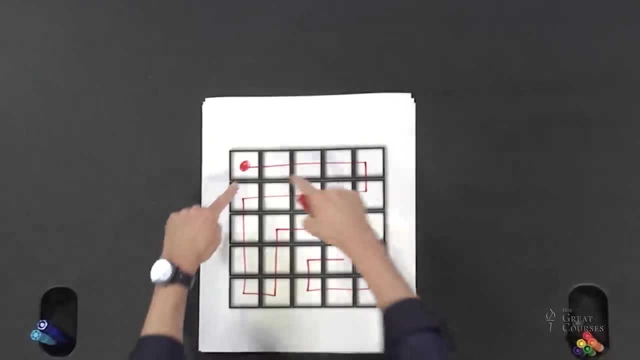 Maybe get a little bit crazy, But I can definitely find a path that does indeed visit each cell exactly once. Great, That was starting from the top left corner. Can I do it from a different position? Well, let's try it, Let's find out. 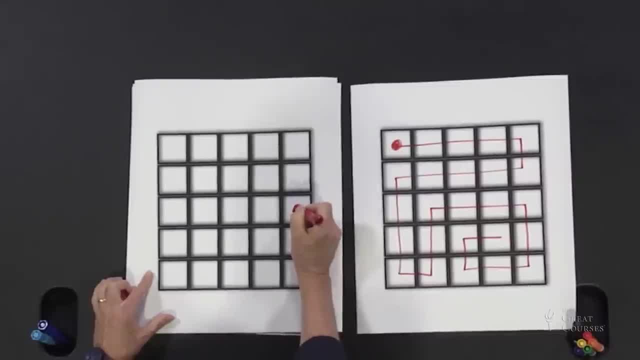 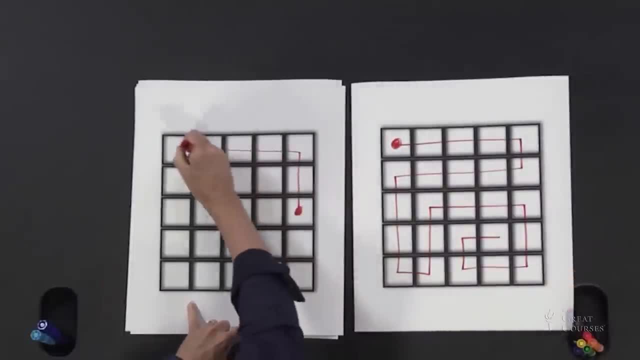 Okay, How about starting from the middle of the side? Can I find a path that visits every cell exactly once? Well, let's try it. Kind of random here, Just get going. I'm going to do something like this, Am I okay? 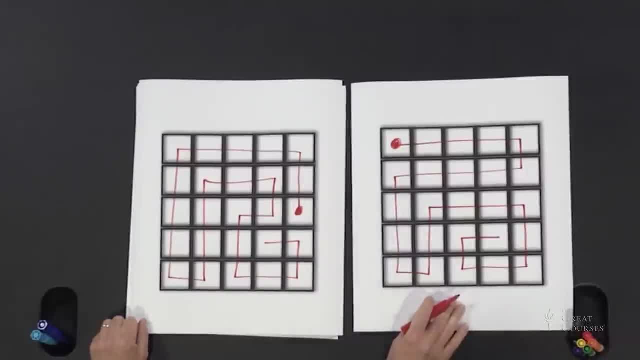 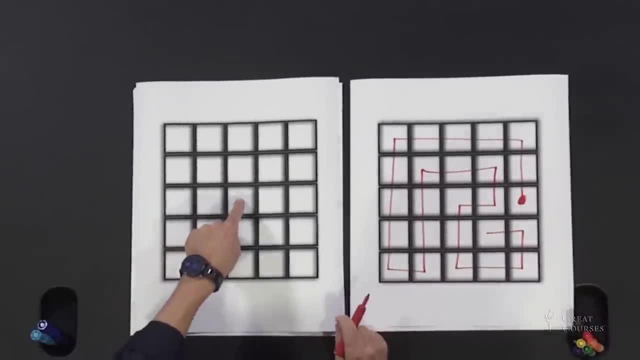 Oh, looking just fine, Great, All right. Loads of fun. So I just kept going. In fact, let's choose another spot, Say I choose the very middle one. All right, I'm going to do it because I think I can see an answer. 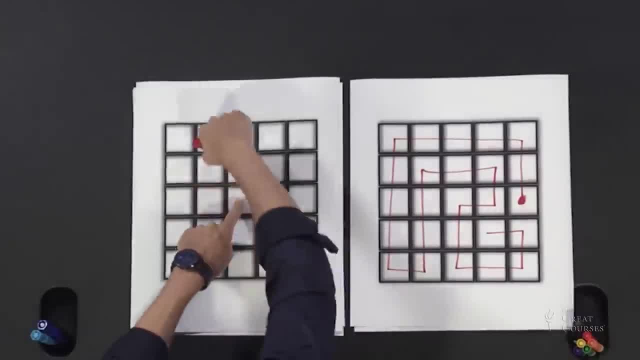 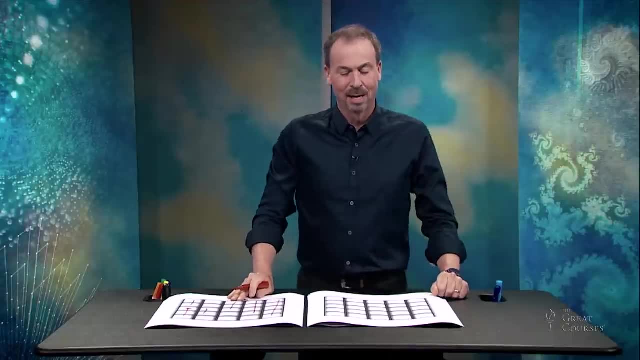 right away. What if I just did a spiral? Can you see that's going to work? Huh, So the middle position works as well. But then here's the thing: I chose a different square, like this one, and matters seem to change. 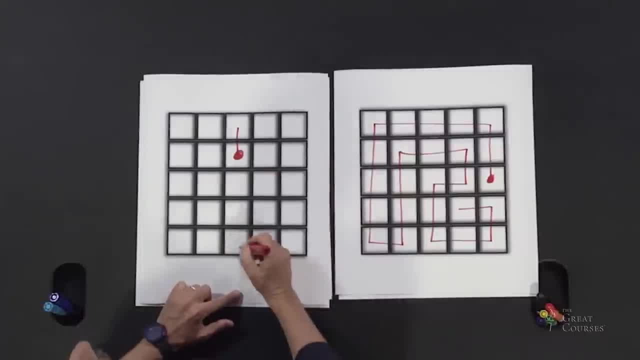 I'm going to try this one, So maybe I'll start by going up. It's a vertical step. Maybe I'll go over And I can do something like this. It looks pretty good. Maybe I'll come down, do a little zigzag. 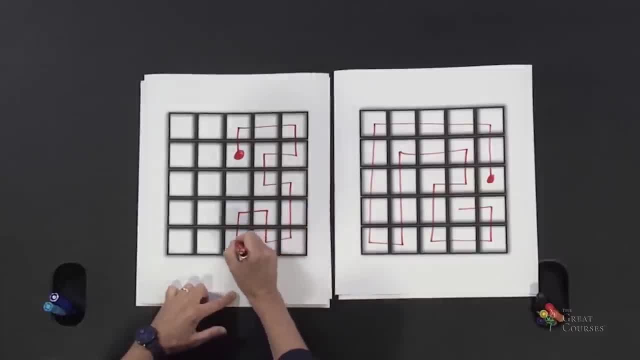 Okay, So far, so good. Maybe I'll come around like this: I'm not nervous yet It looks fine. Ooh, Now I'm getting a bit nervous, So I go up here. I've got to get to that cell and not miss it. 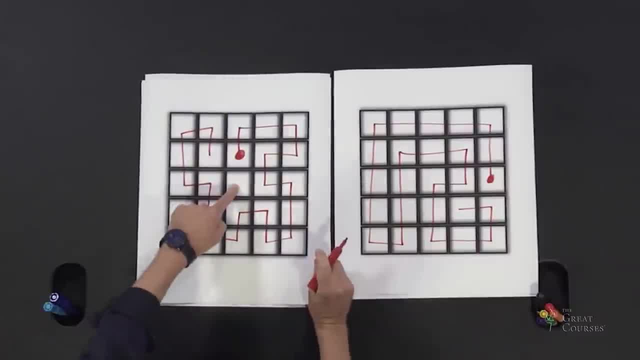 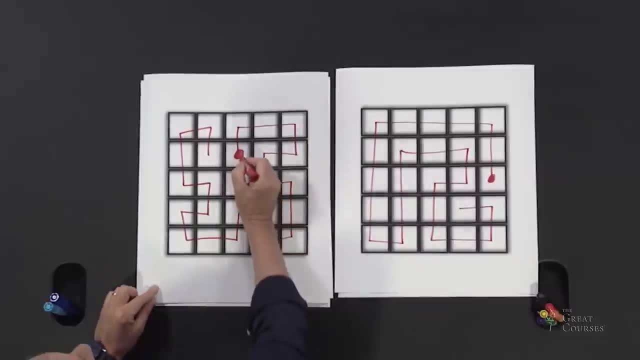 But I've got all these over here, So maybe I'll do them, but then I'm stuck. I could do a diagonal step, but I won't allow that. My game was only vertical and horizontal steps. So this cell, this one, I guess what is it? 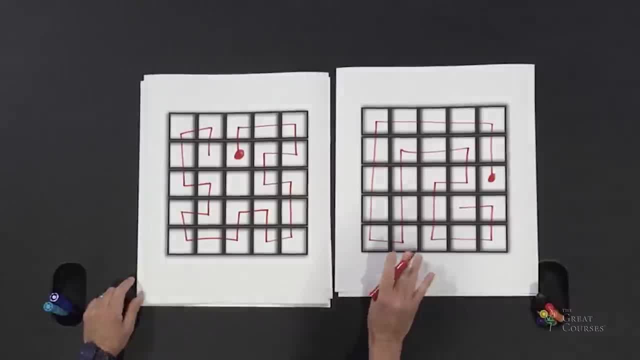 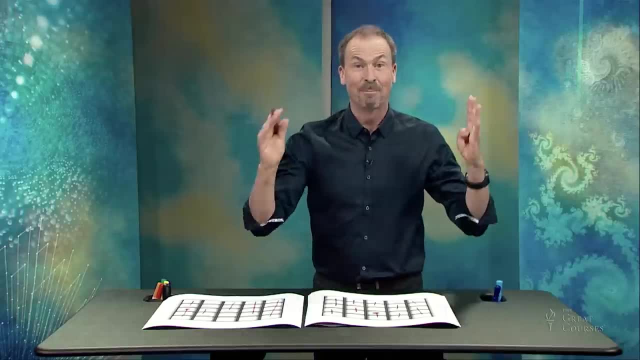 one in from the middle was questionable. In fact, I tried it lots of different ways. Maybe I'll do something more like this, And I seem to get stuck. In fact, as a young lad, as I kept doing this, I always got stuck on that one. 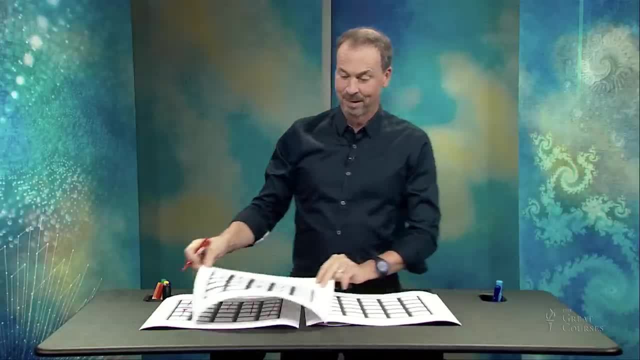 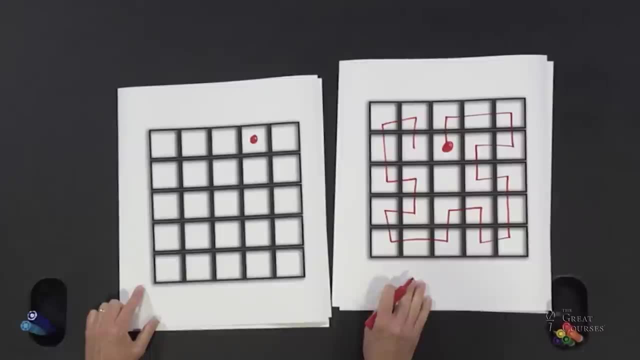 Well, let me try another one. Are there other cells that make you stuck, For example? let's try I don't know this one here. We haven't done that one yet. Well, let's do it, Give it a go. 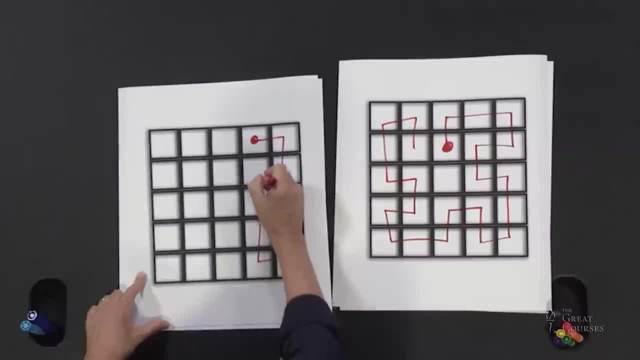 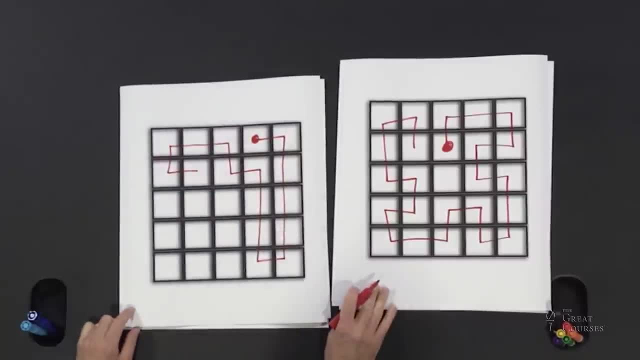 See what happens. So this feels fine so far. So I've got that half of the board done, or that two-fifths of the board. Maybe do something like this and get this portion of the board done. Looks good so far actually. 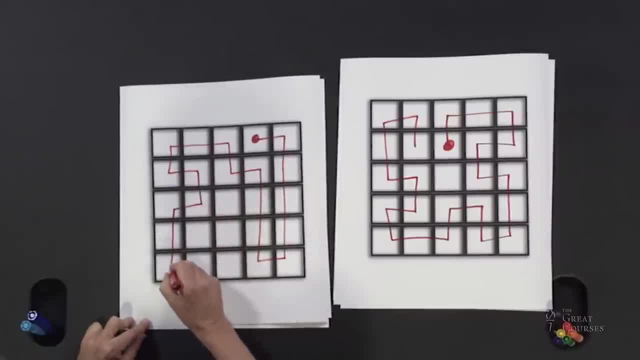 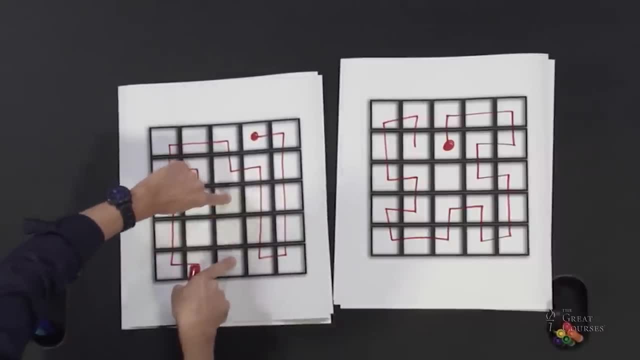 This is great, Let me keep going. Ooh, now I'm starting to get nervous because I kind of want to do something like: either go up here and then I come over and I've got a choice: left or right. 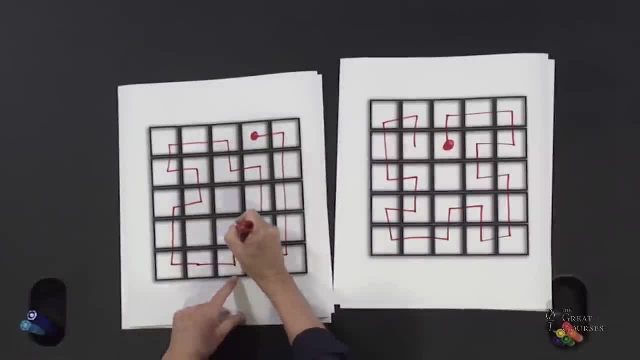 and I'm going to get stuck. So maybe I should do this. But then I'm forced to go up there and I've got a choice again. I'm going to get stuck. I can go one way but not reach the other way. 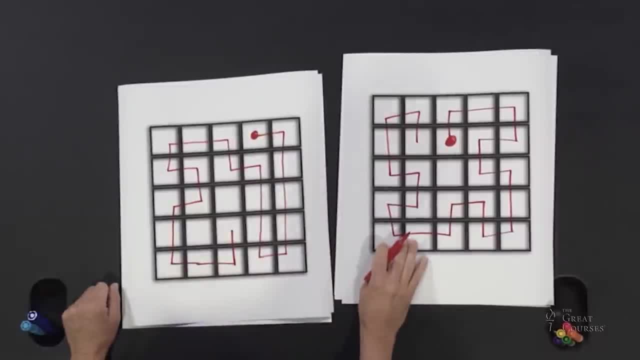 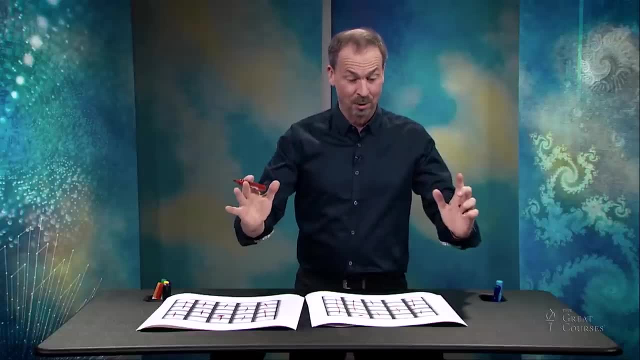 Hmm, So this cell here is troublesome as well. All right, So now let's be a little systematic here. Some cells would definitely- yes, I could do it, because I did it, In fact we've done it here. 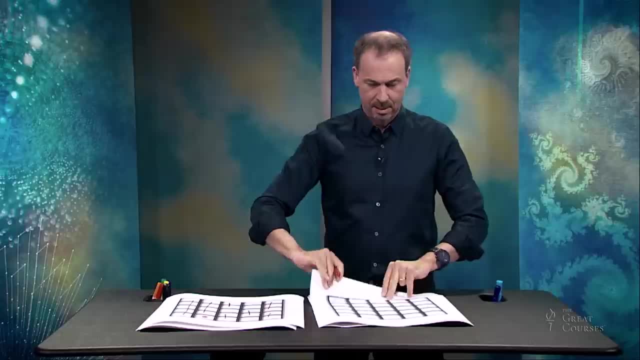 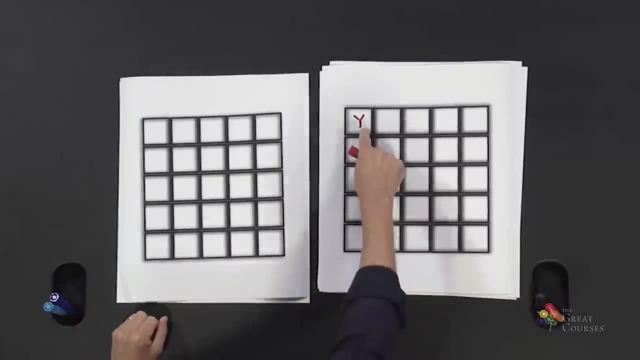 So let me get a clean grid yet again, And what I'll do now is I'll be a little systematic and mark the cells that were yeses, For example, that cell. that was the very first example we tried. yes, we definitely could find a path. 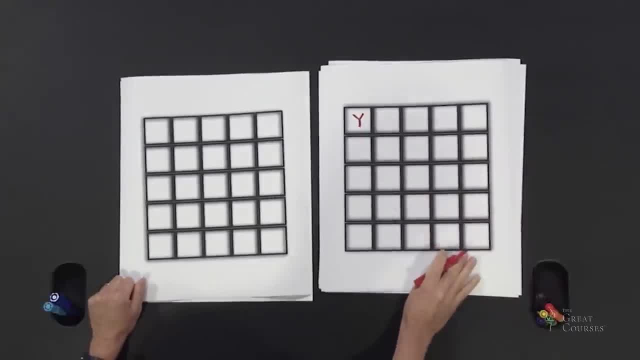 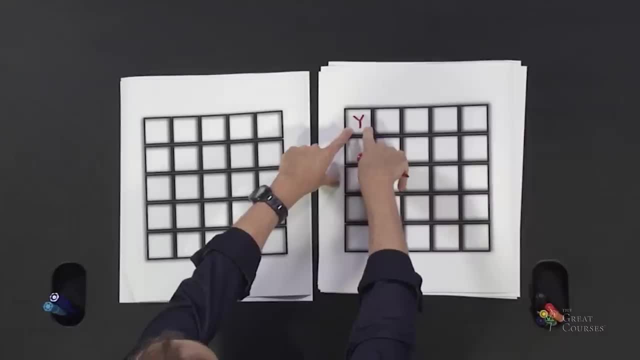 visiting every cell exactly once, with horizontal and vertical steps starting there. Ooh, Actually, let's be clever, We answered this corner cell as a yes. What about this corner cell? Must that be a yes as well? Well, if you think about it, 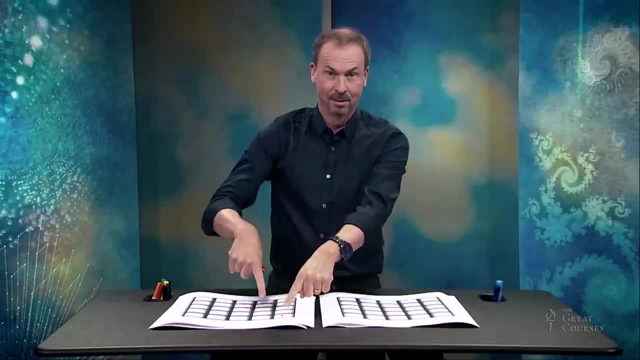 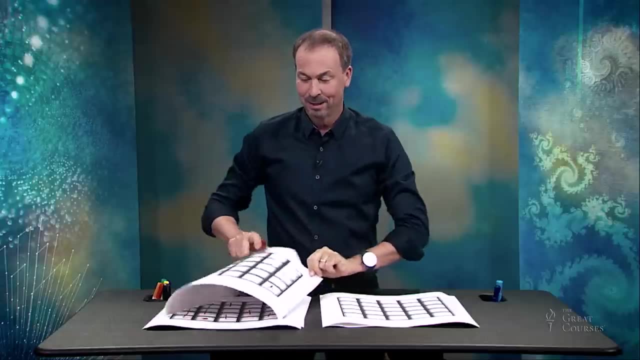 actually yes. Whatever solution we have here, just take your solution and turn it around 90 degrees, and that would be a solution for the top right corner. So if the top left corner is a yes, the top right corner must also be a yes. 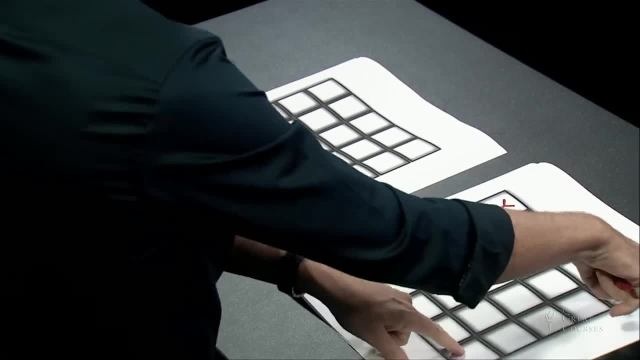 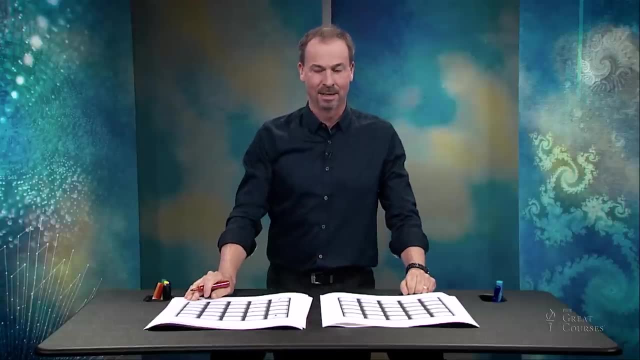 Oh, and then take that solution and turn it another 90 degrees. That means this corner is a yes as well. In fact, all four corners must be yes cells, All right, So definitely four corners are yeses in this picture. 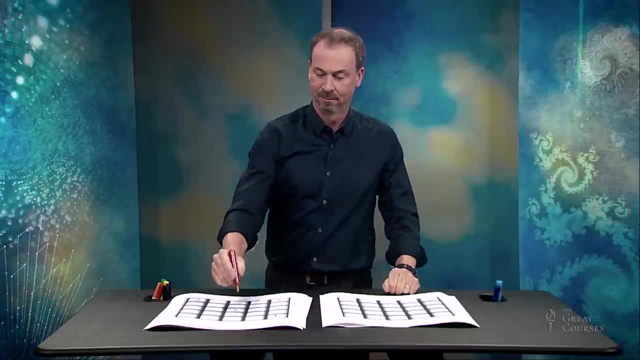 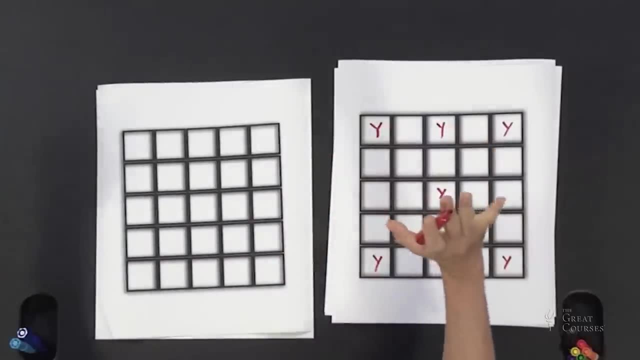 We did the middle cell next. That was a yes, We actually did it. That little spiral was fine. What else did we do? We did the middle cell of a side, if I remember. So that was a yes, Ah, but then by symmetry again. 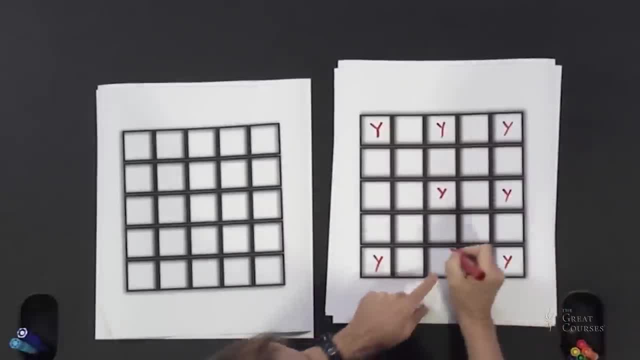 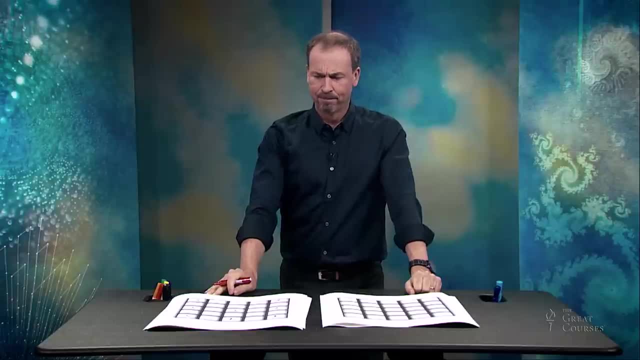 rotating 90 degrees means this was a yes, this was a yes and this was a yes. All right. Well, that looks pretty. Are there any more yeses in this picture? Hmm, Well, right now we do have a couple of question marks. 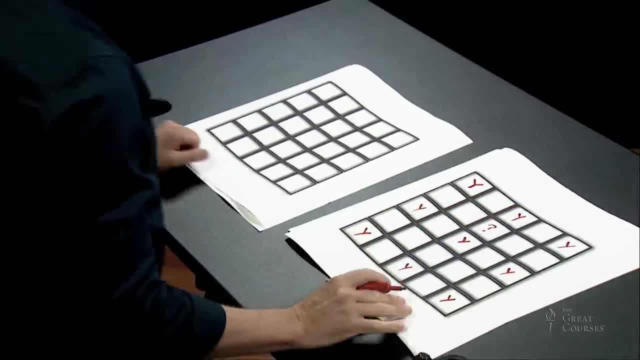 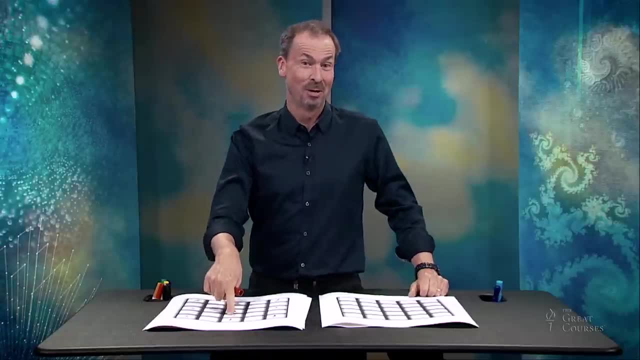 Now we tried this one, and I only tried it once today, but I actually tried that cell for years as a kid and I could never do it. But I must have been a strange child, because I never actually said the answer is no. 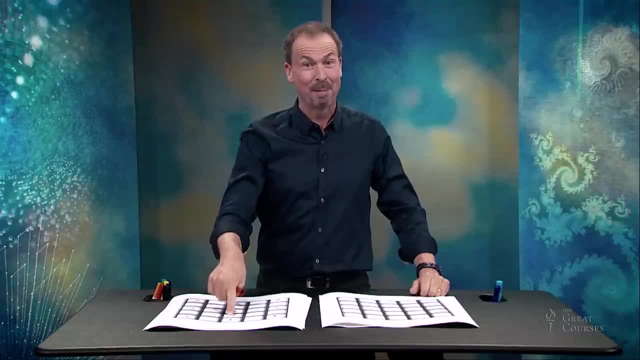 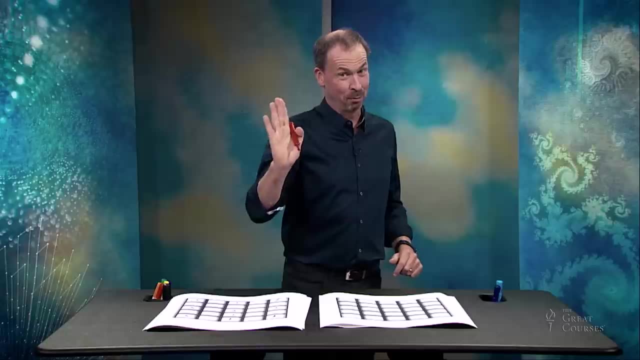 because I realized maybe I just didn't try hard enough, If I kept going, maybe I'll stumble upon the solution eventually. So I just was honest and said: this is still a question to me. My gut told me it's probably a no cell. 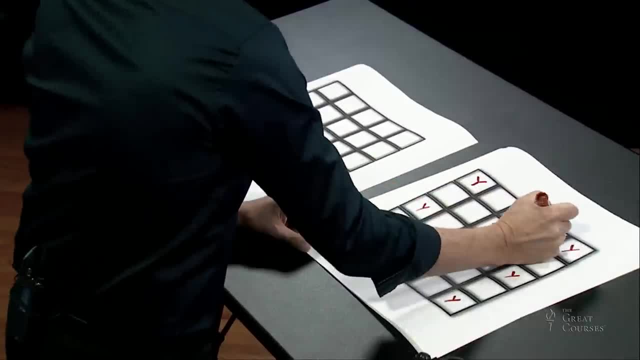 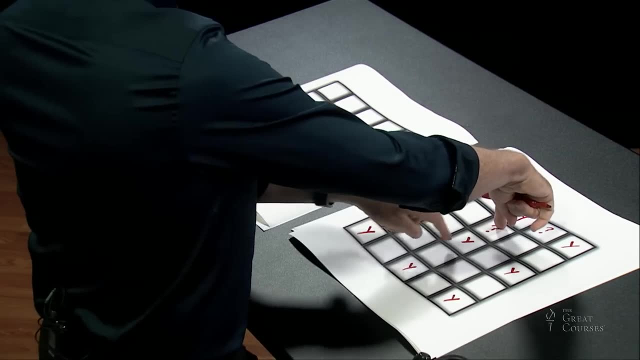 but I put a question mark nonetheless. Also, we questioned this one. I think we tried that one earlier, So that was a questionable cell as well. Oh then, by symmetry, if this cell is questionable, rotate 90 degrees means that this cell is also questionable. 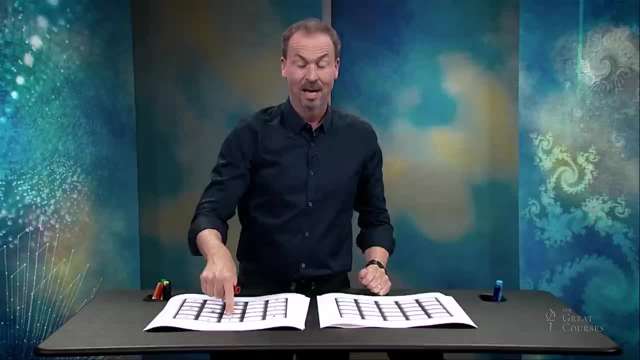 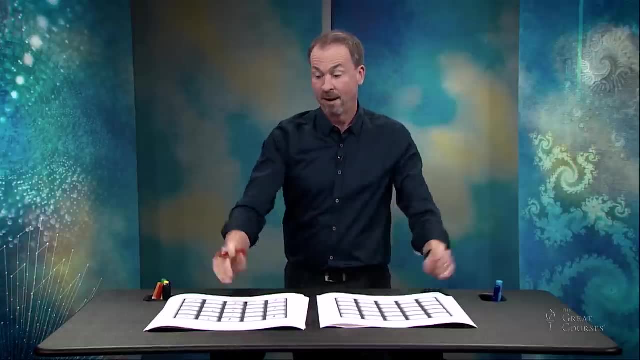 Because I've had a solution for this one. just rotate it 90 degrees back, and I would have had a solution for that one as well. In fact, I can argue, all of these four cells here are questionable, In fact. again, 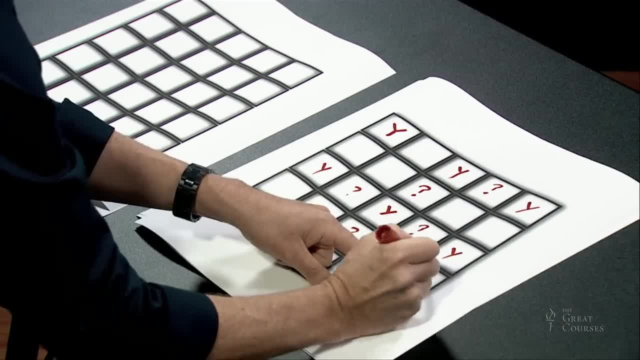 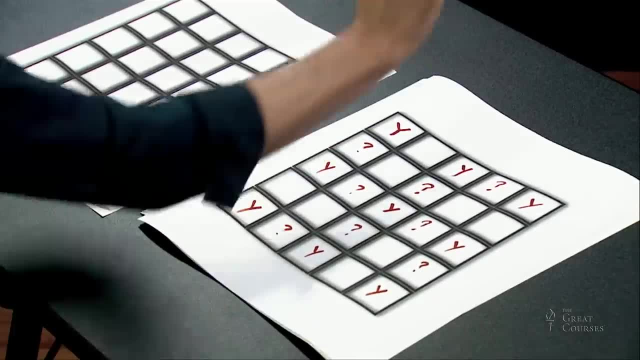 90-degree rotation of this one gets me where is it Here? So that must be questionable. 90-degree rotation: questionable and questionable. Now I'm starting to fill in the grid. Oh, actually I'm going to do more symmetry. 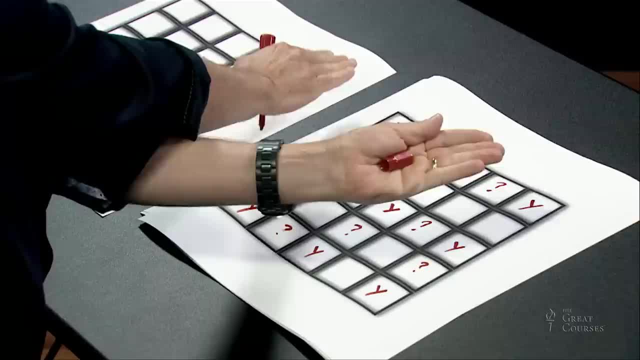 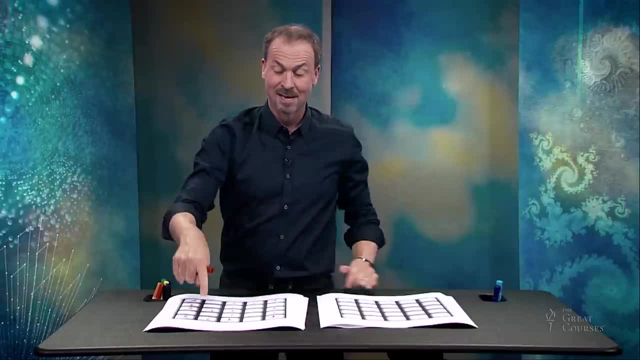 If this cell is questionable, I bet if I just reflect the image, this cell must also be questionable, Because if I had a solution here somehow, then I'll just reflect back and that would have given me a solution there. So this cell must also be questionable. 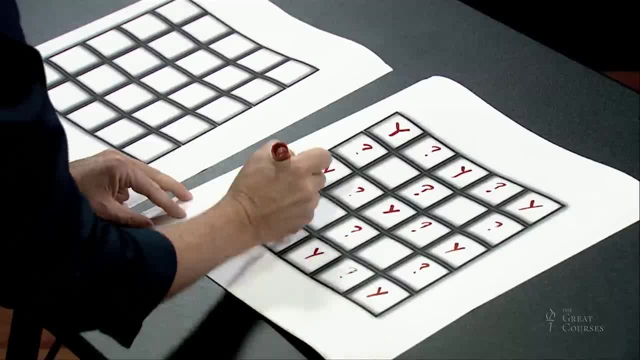 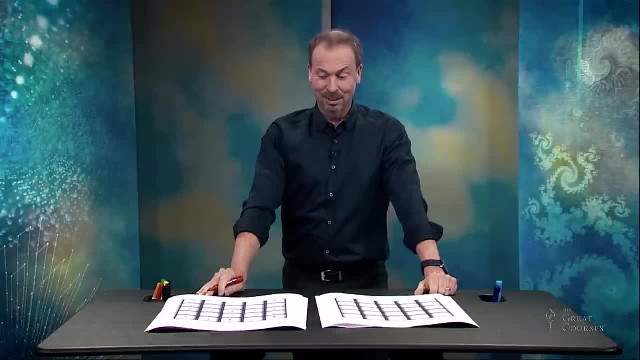 And I guess by 90-degree symmetry. all the side cells that are left over are also questionable. All right, okay. So then I was doing some systematic work here, but we see these four cells we haven't tried yet. All right, can they be done? 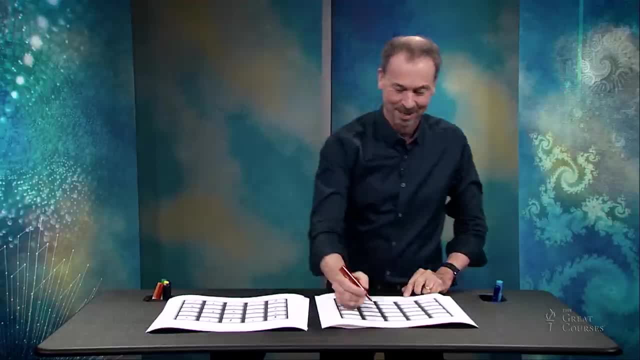 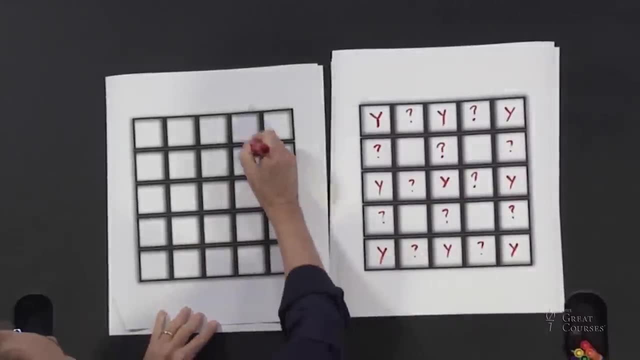 or can they not be done? Well, let's try it. So I'll start here. That's the right one, isn't it? Yep, And see if I can do a path that visits every cell exactly once, with vertical and horizontal steps. 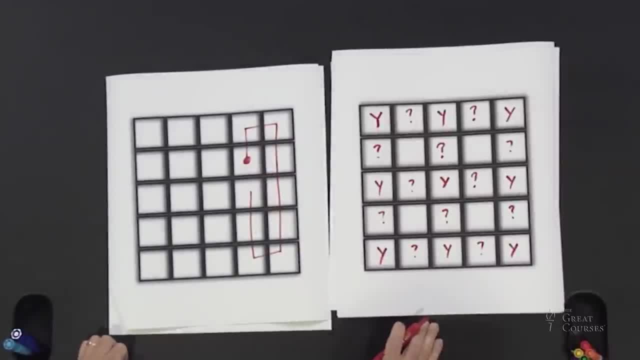 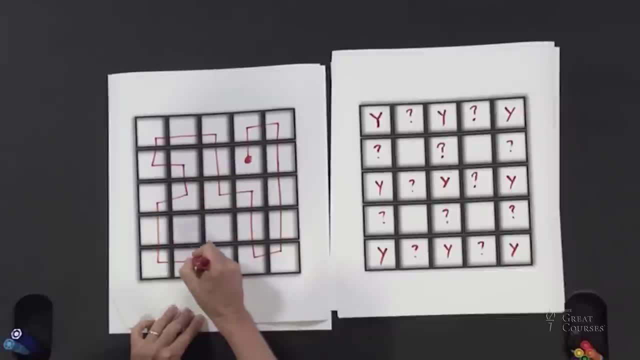 And I'm just trying it out here, Not sure where I'm going. So far, no pickles, Everything's looking fine. Do I look? okay? Look at that, It can be done. That's a yes. By rotational symmetry. that's a yes. 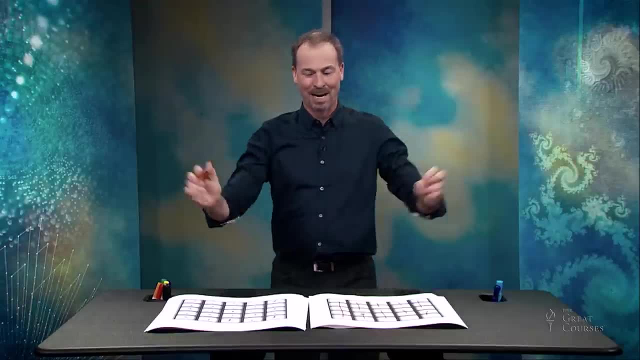 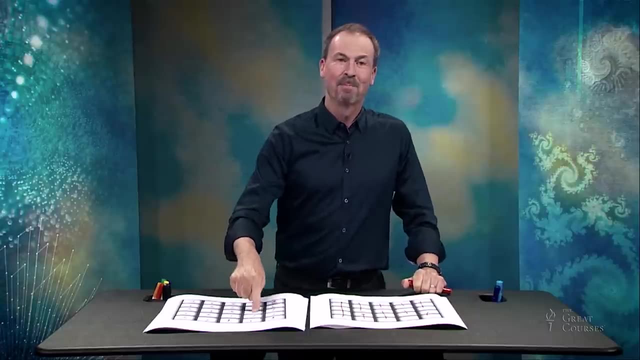 That's a no, That's a yes, That's a yes. All right, I know for sure that these Ys are definitely yes cells, because we actually did it. But the puzzle for me was: are these questionable cells actually just questions? 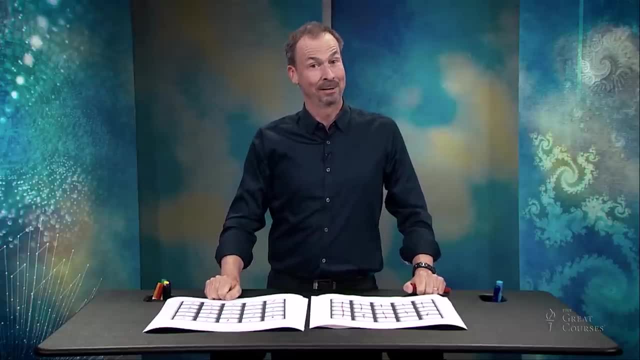 Could they be done if I tried harder? Or are they really nos? And that is the question that stuck with me for years. Are they really no cells? My gut was telling me they really were, because I tried it lots, and lots and lots and lots of times. 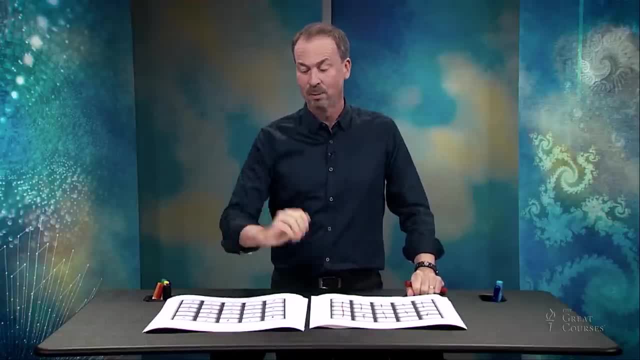 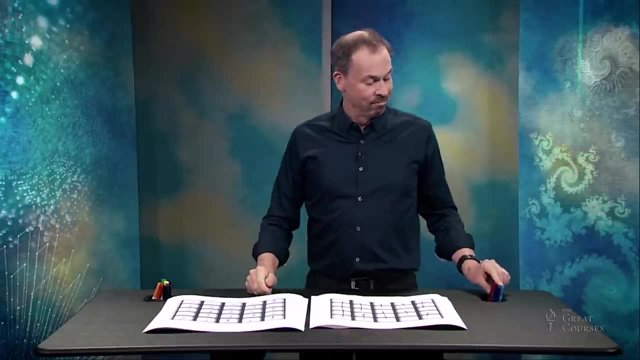 I can never do it, But I wanted the logic behind it. Why would they be no cells? Maybe I just need to try one more time. Okay, So that question stayed with me for I don't know, a good six or seven years. 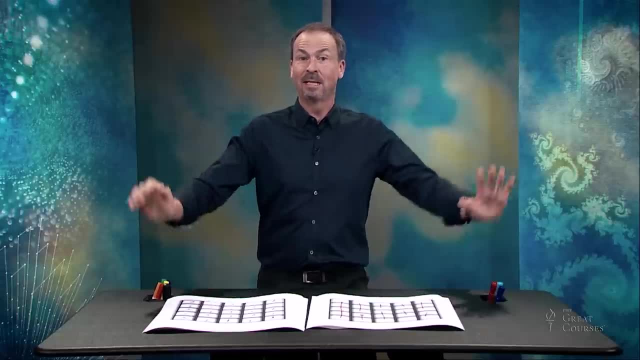 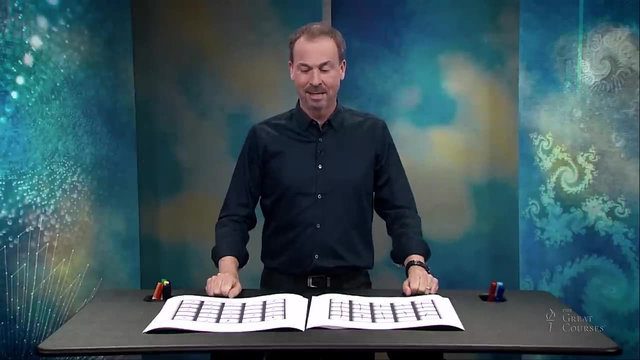 And I remember walking to school in grade 10 one day, not particularly thinking about this problem, and a strange, wondrous epiphany just hit me Out of the blue. I suddenly saw a logical reason why these question marks had to be no cells. 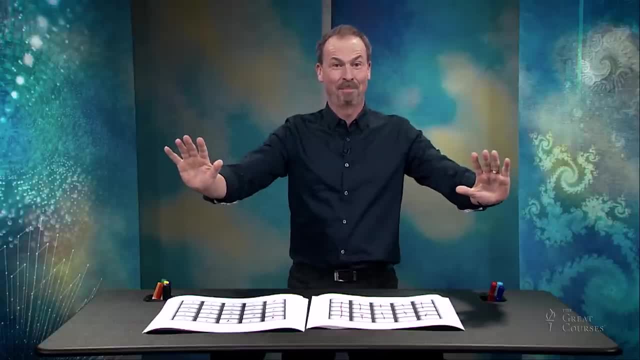 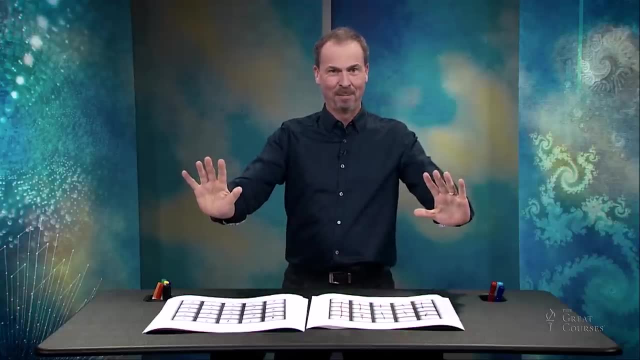 So I'm going to give away my epiphany now. I'm going to give away the result. that just makes it glaringly obvious why these are nos Okay. So if you want to wait for the epiphany yourself, maybe you want to pause for a moment. 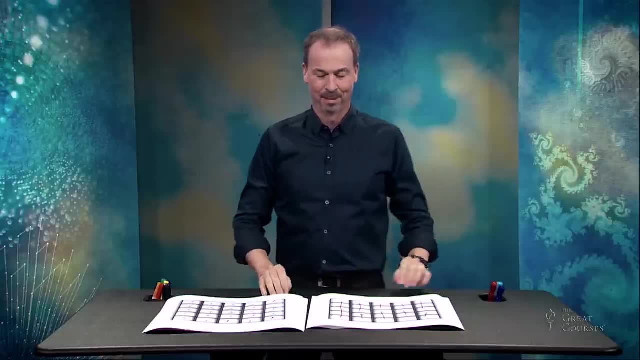 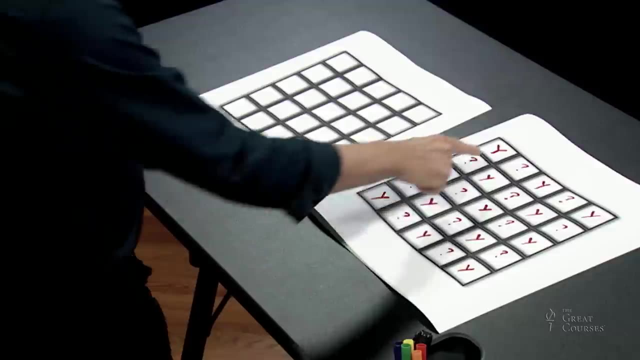 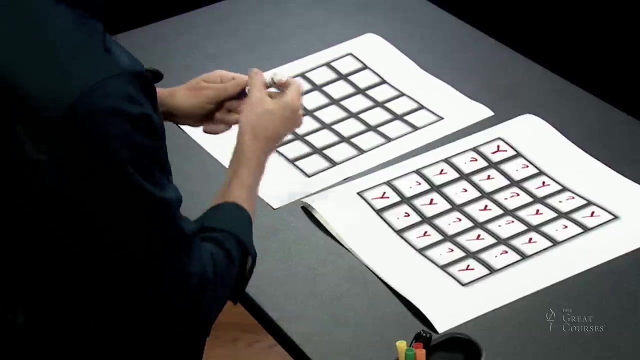 and just go for a walk or something, because I'm about to give it away, Right? Fair warning. So look at what we've got here. Have you noticed that the Ys and the question marks make a checkerboard pattern? Hmm, In fact, let me really make it obvious. 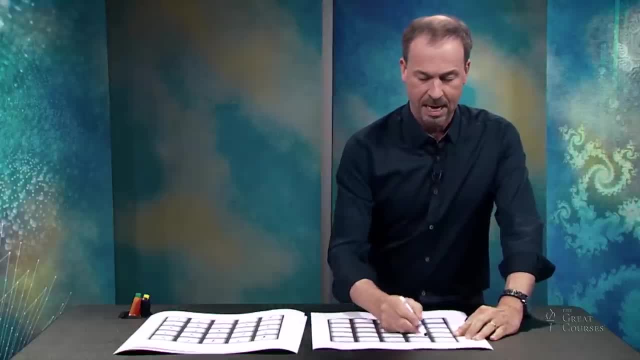 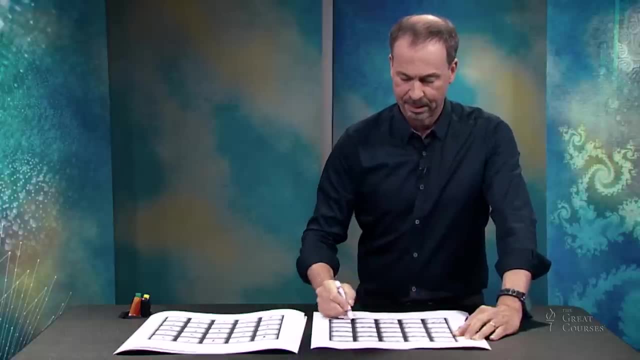 A checkerboard pattern, So I'll actually color in some cells just like a checkerboard. So I've got some purple cells and I'll have some white cells. All right, And look at that, How many purple cells are there? Well, let's count them. 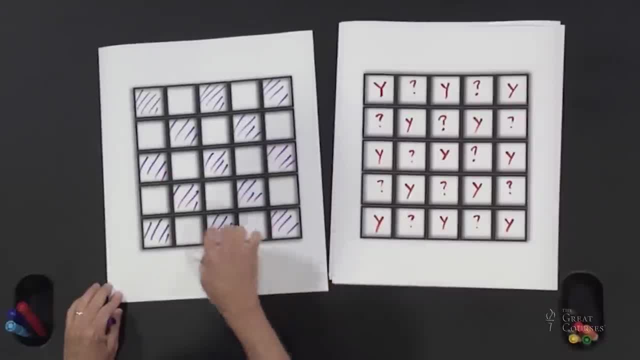 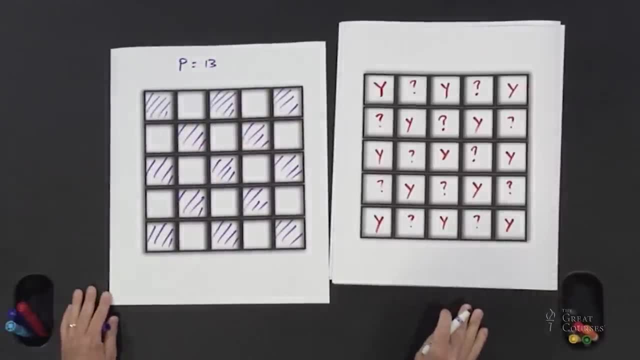 One, two, three, four, five. One, two, three, four, five. That makes 10. And one, two, three. So the purple cells number in 13. And the white cells then must be 12 of them. 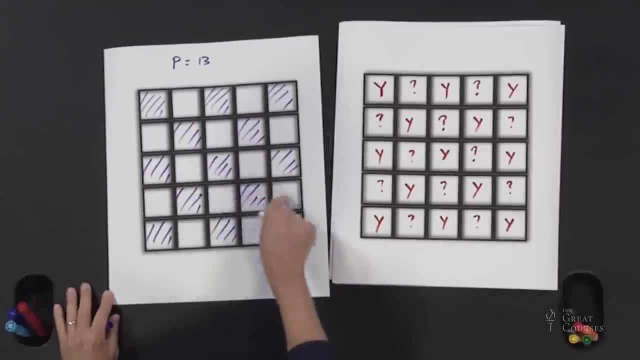 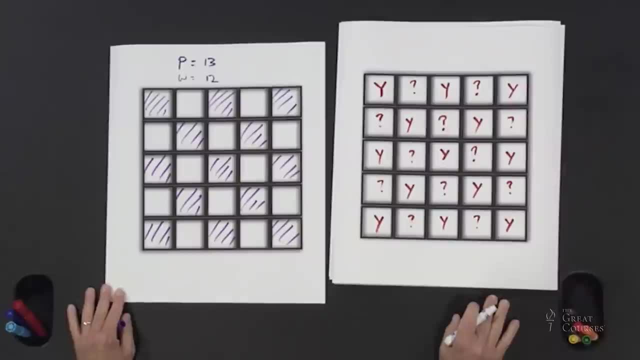 because there's 25 cells in all: One, two, three, four, five. One, two, three, four five, One, two. The white cells come in 12, a set of 12.. All right, So what? 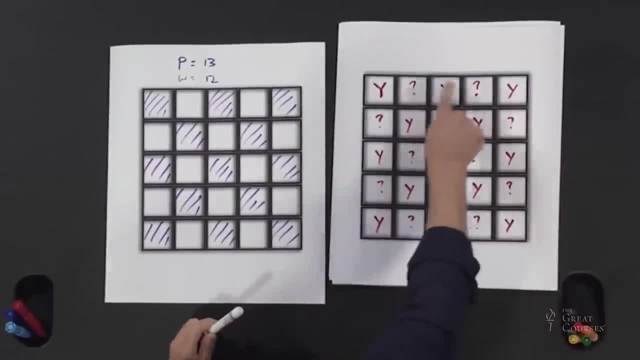 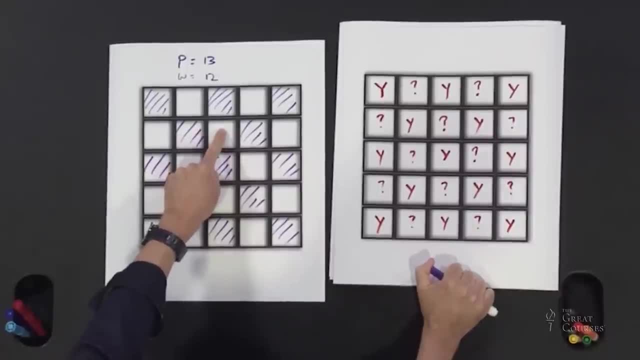 Well notice: all the question marks are in the locations of these white cells. So I'm wondering: why would it be impossible to start a path on a white cell? So let's think about it. I'm on a white cell, So maybe my first cell is white. 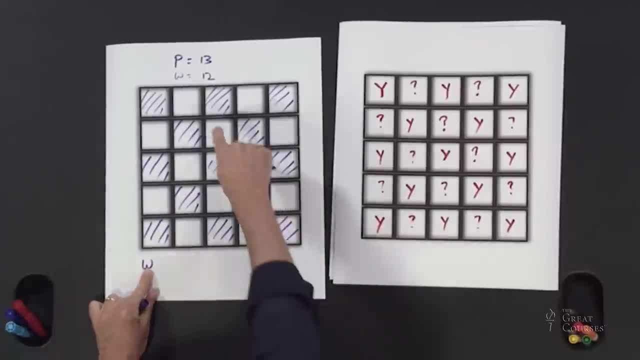 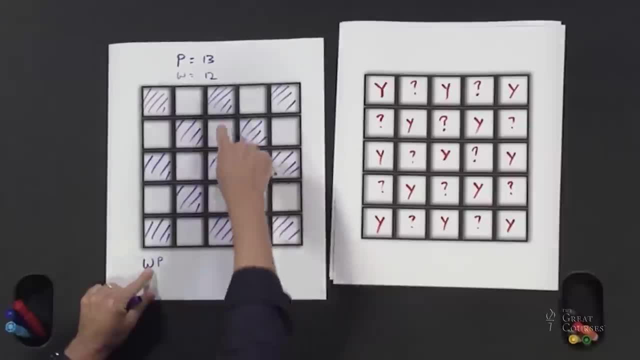 I'll actually write down W, for my first cell is white. Whichever white cell I'm in, I've got no choice but to next walk into a purple cell. whichever direction I go, the next cell has to be purple. Okay, If I'm in a purple cell. 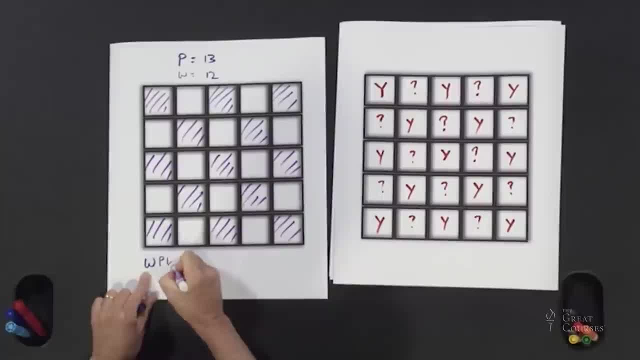 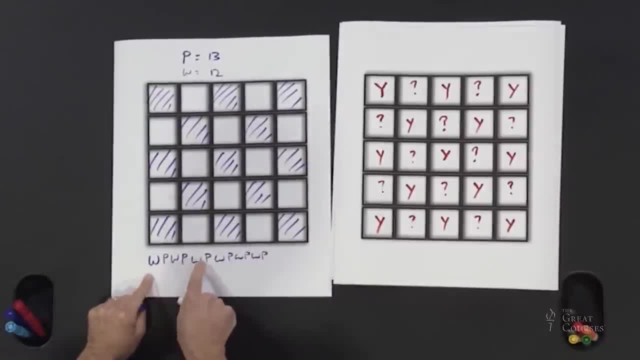 then white, then purple. Okay, How many steps is that? One, two, three, four, five, six, seven, eight, nine, 10,, 11,, 12.. Okay, It's only 12 of the steps. 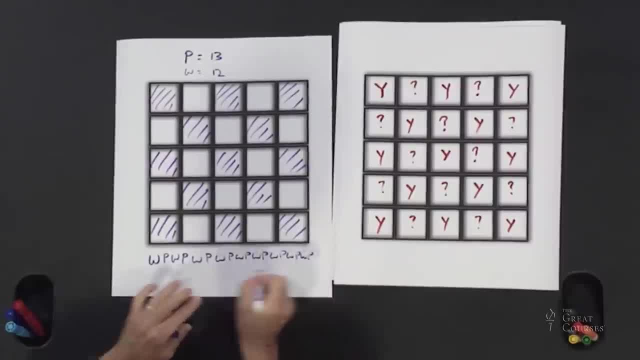 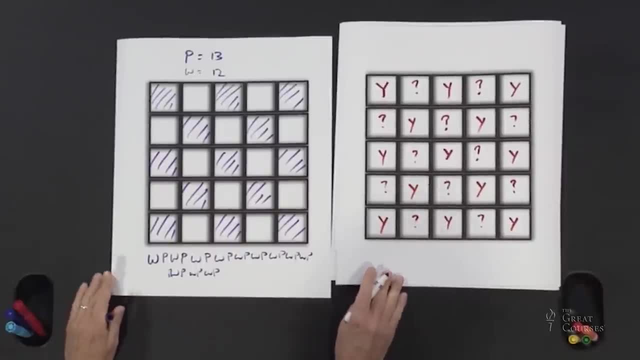 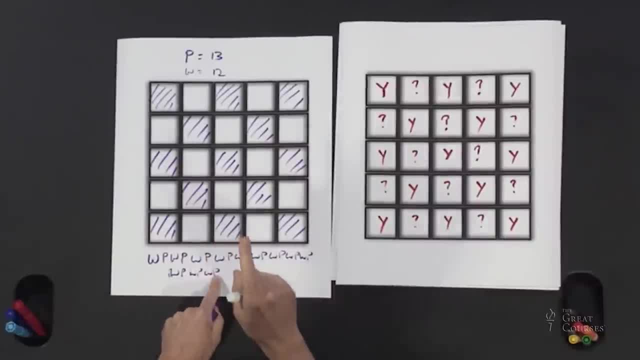 I'm currently in a purple cell and I have to take one more step, but we have a problem. Look, There are 12 white cells and 13 purple cells, And right now I've used up one, two, three. 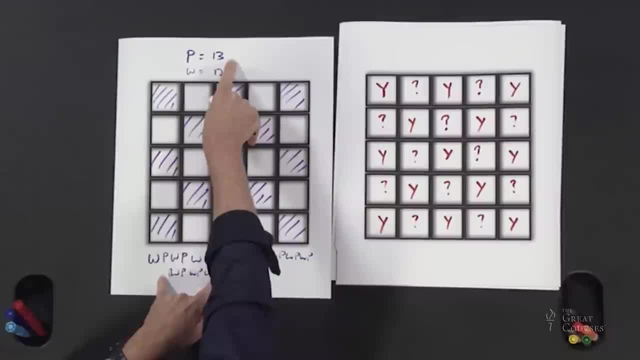 four, five, six, seven, eight, nine, 10,, 11,, 12 whites, and I've only used up 12 purples. We still have an extra purple to go, which means I'm in a pickle. 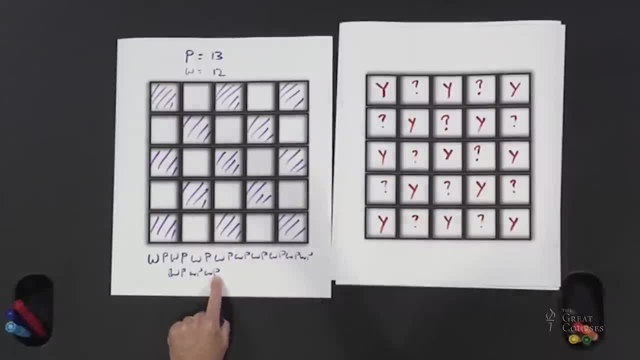 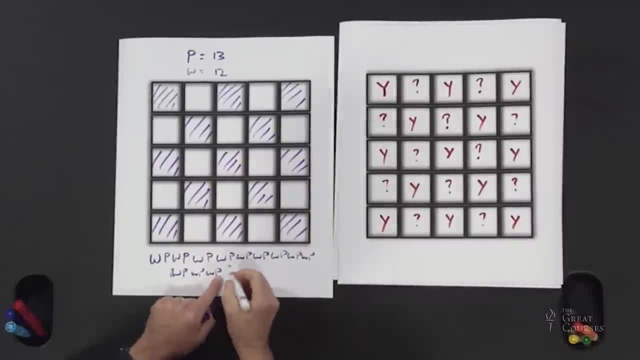 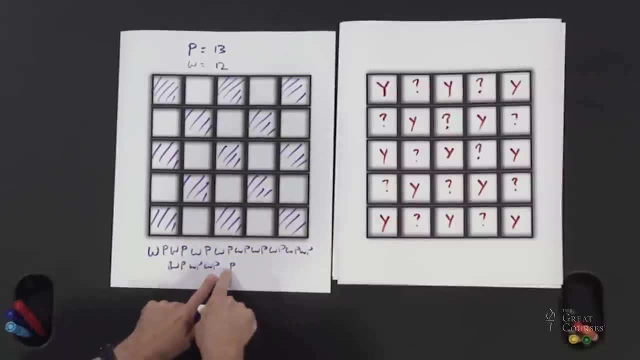 and I've only got a purple to use. but it can't be purple. but it can't be purple, because if it's purple I'm in trouble. I'm meant to go to a white cell next. That's impossible. You cannot start in a white cell. 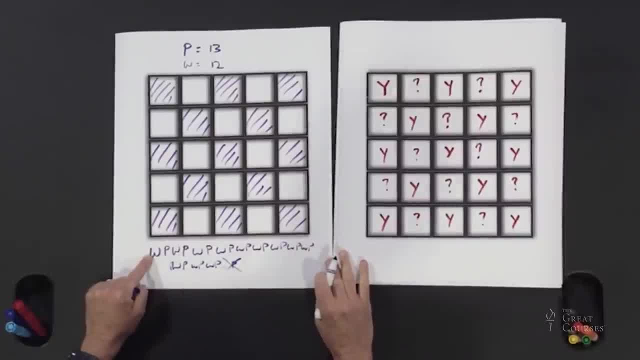 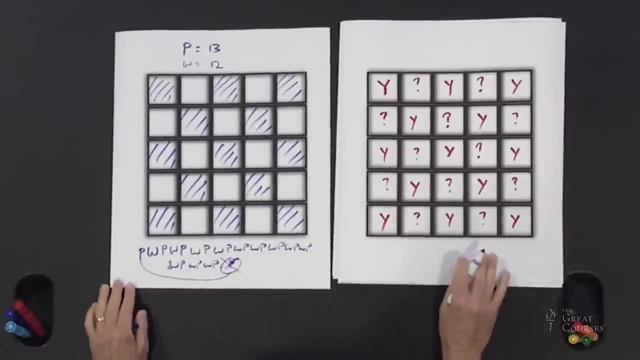 because you've run out of the white cells before you used up all the purple cells. But the only way this puzzle could possibly work is so that extra purple cell is so that extra purple cell appears at the beginning. appears at the beginning For this puzzle to work. 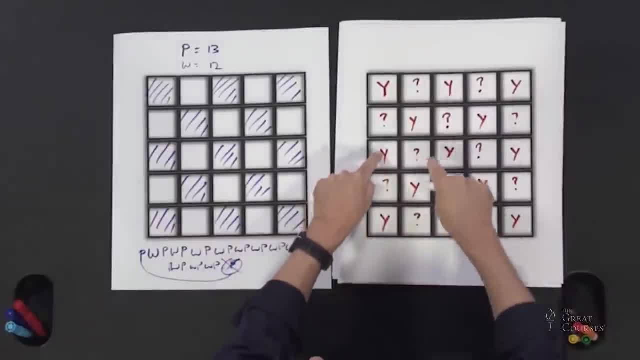 you must start on a purple cell. you must start on a purple cell and look: Indeed, we could do it if we did. Indeed, we could do it if we did. Isn't that beautiful? Isn't that beautiful? That was an epiphany. 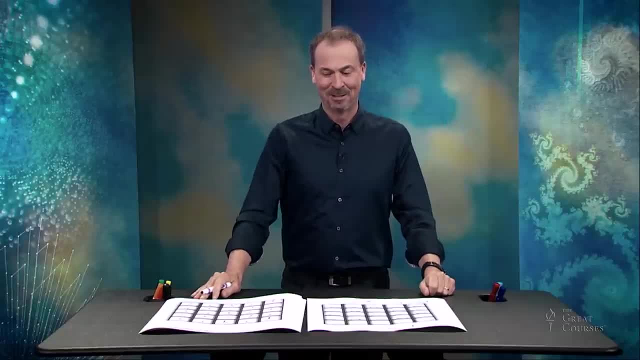 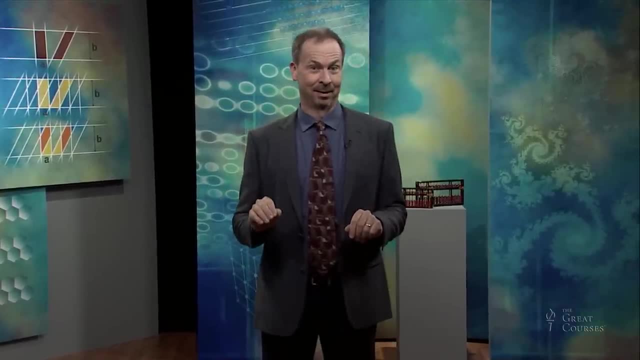 That made me say, wow, there's something going on in this universe, It's just beautiful. going on in this universe, It's just beautiful. Okay, we're still only scratching the surface of things. the surface of things, Let's push play. 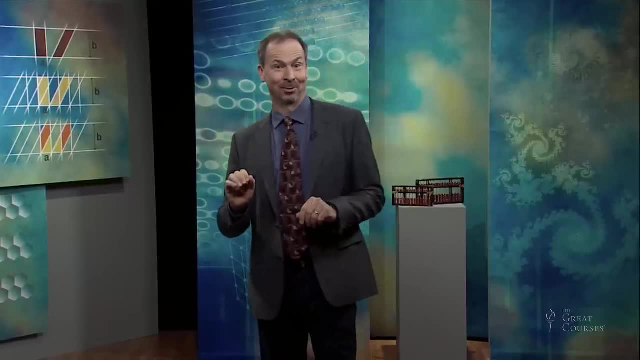 with this 5x5 grid even further. There are more surprises in store. There are more surprises in store, But this time let's view the 5x5 grid as an array of dots. as an array of dots Now. 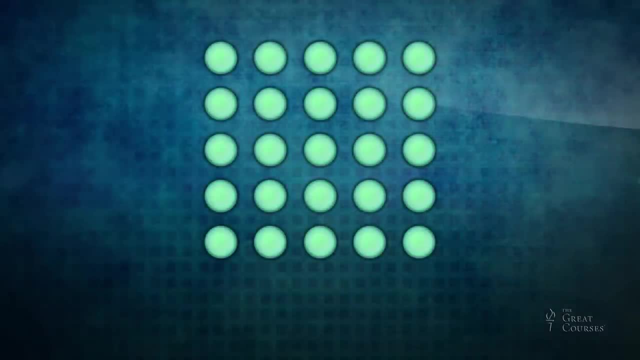 stare at this picture. It is certainly a picture of 25 dots, of 25 dots, But can you see in this picture the sum 1 plus 2 plus 3 plus 4 plus 5, the sum 1 plus 2 plus 3 plus 4 plus 5? 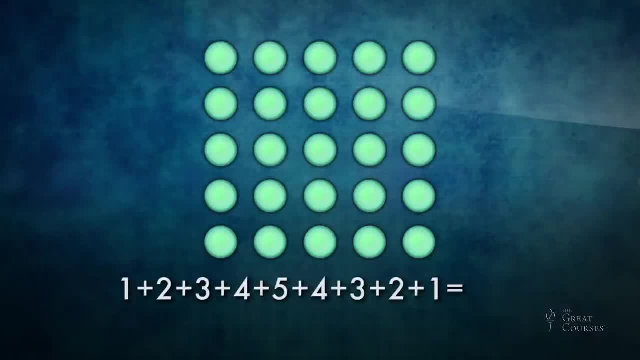 plus 4 plus 3 plus 2 plus 1? plus 4 plus 3 plus 2 plus 1?. Now it takes a moment, It takes an epiphany: Here goes, Here goes. Look at the diagonals. 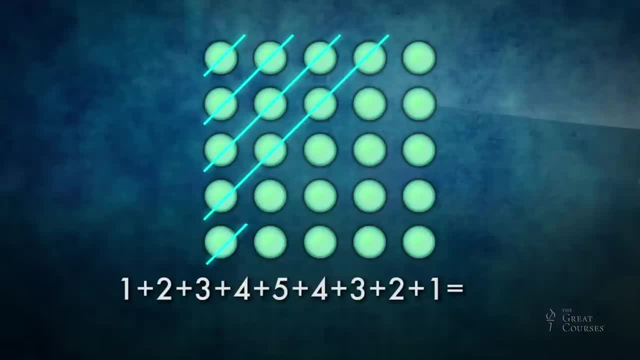 Look at the diagonals 1,, 2,, 3,, 4,, 5,, 4,, 3,, 2, 1.. The sum we seek matches the diagonals of the square. There are 25 dots in all. 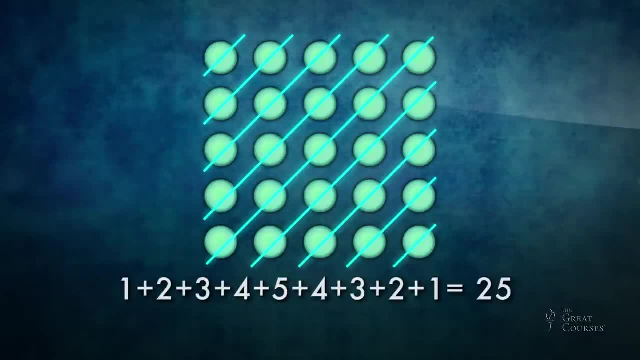 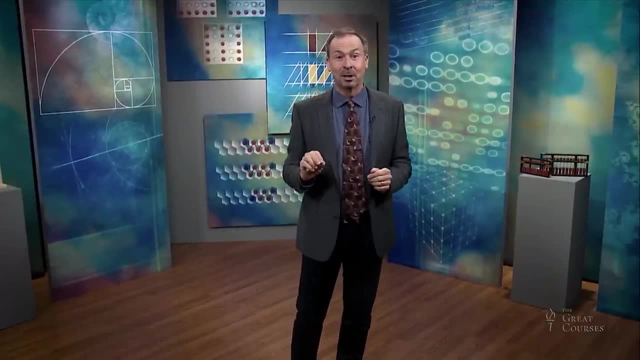 So, without doing a lick of arithmetic, we can say: the value of the sum must be 25.. I love this. I love this. This picture is powerful, It's literal self. What is the sum of the numbers 1,, 2,? 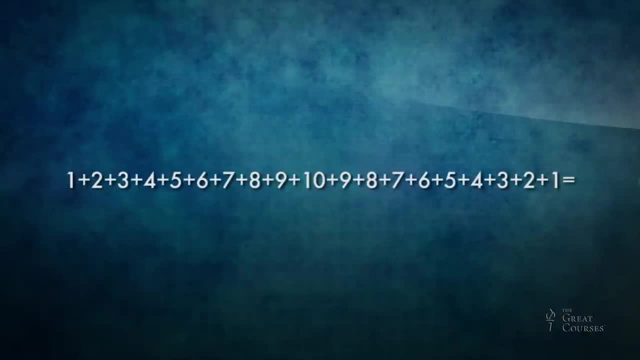 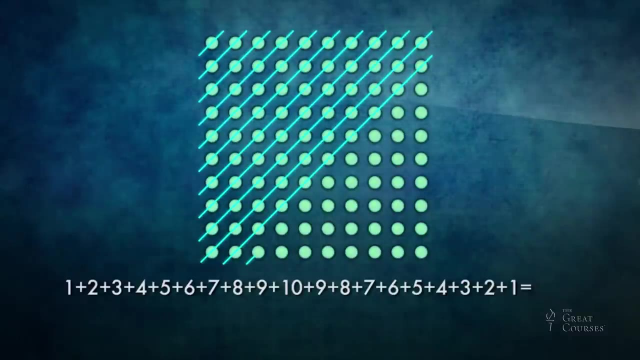 3, all the way up to 10 and back down again. Well, this sum must come from the diagonals of a 10 by 10 array of dots And, again, without a lick of arithmetic, the value of the sum must be: 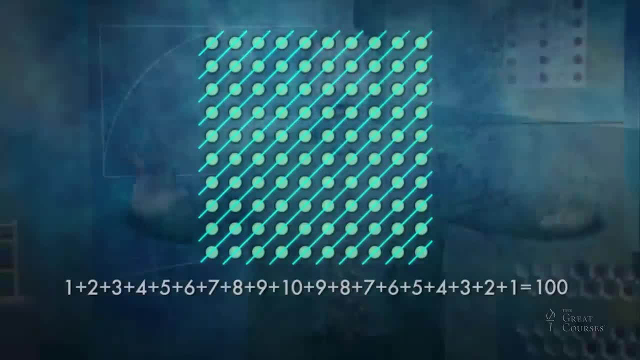 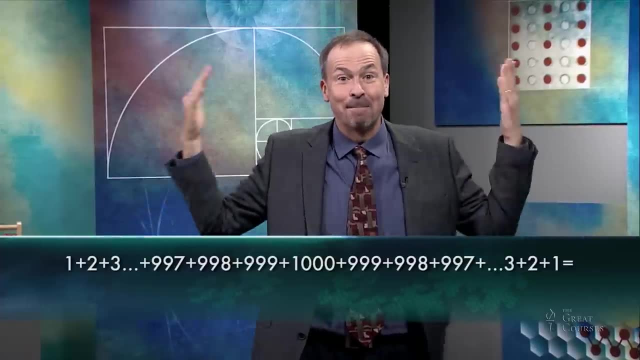 10 squared 100.. So OK, here's the power. What is the sum of all the numbers from 1 to 1000? back down again. Well, it must be 1000 squared from 1000 by 1000. 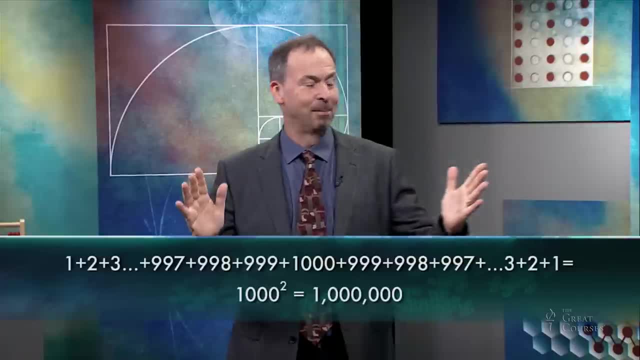 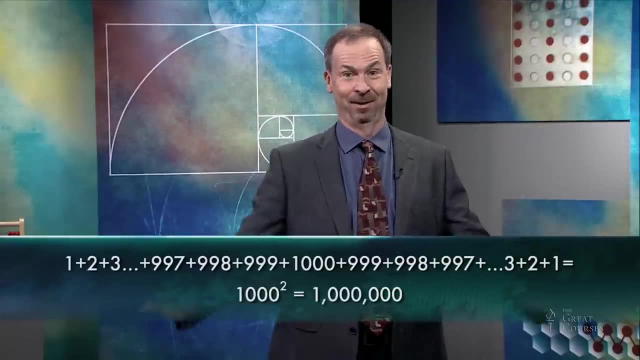 array of dots: 1000 squared is a million. Imagine trying to compute that on a calculator: 1 plus 2 plus 3 plus 4, all the way up to 1000 and back down again. It would take forever The picture here. 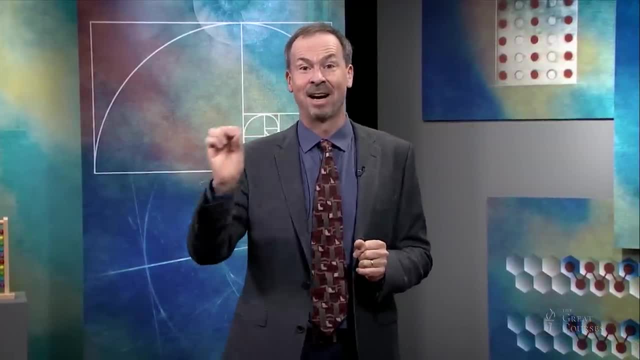 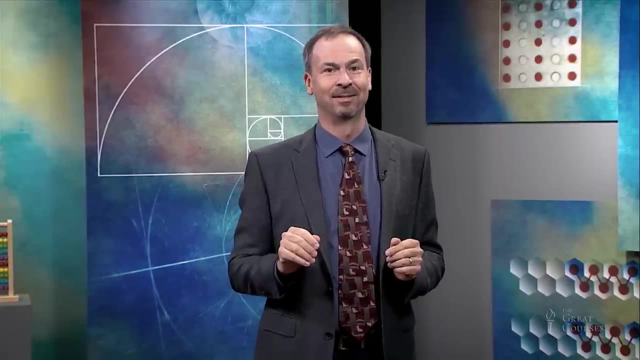 is mightier than the machine. The answer is available to us in the blink of an eye via this picture. The sum of all the numbers is 10 squared from 1000 by 1000. array of dots: OK, so what? Who cares about these sums? 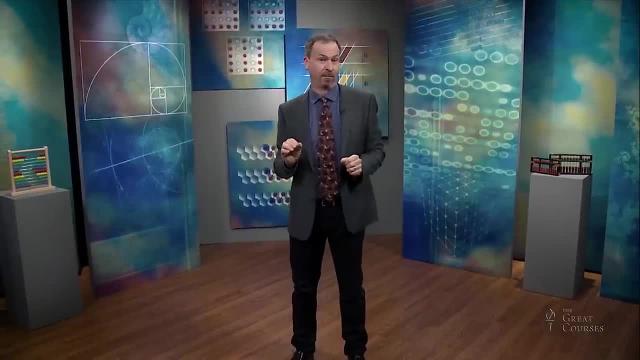 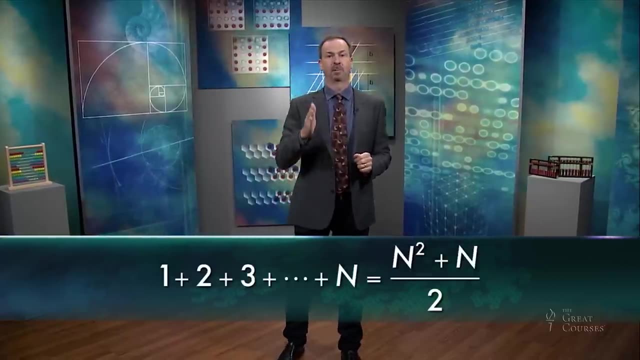 Well, actually school curricula do. In my high school days we had to memorize a general formula for the sum of numbers. The formula looked like this: The sum of the first n numbers, 1 plus 2 plus 3. 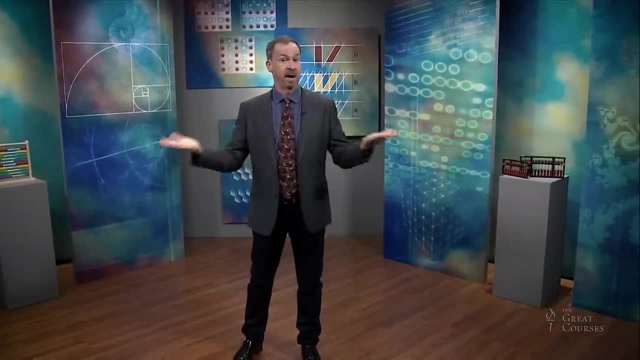 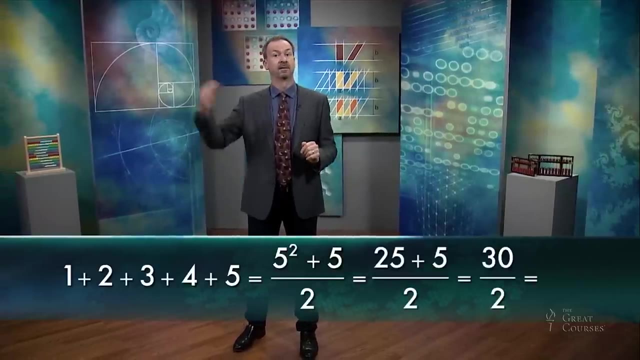 all the way up to sum number. n is n squared plus n, all divided by 2.. For example, 5 squared plus 5, 25 plus 5, that's 30. then divided by 2 is 15.. And one can check that 1 plus 2 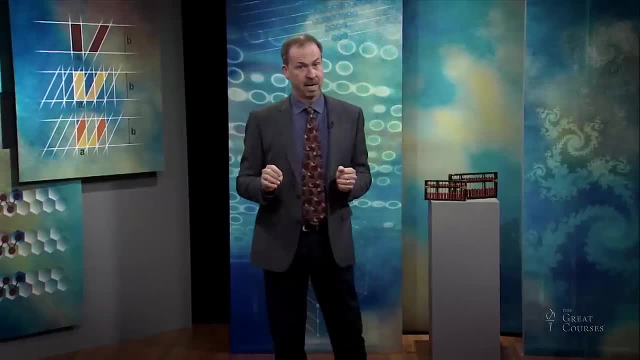 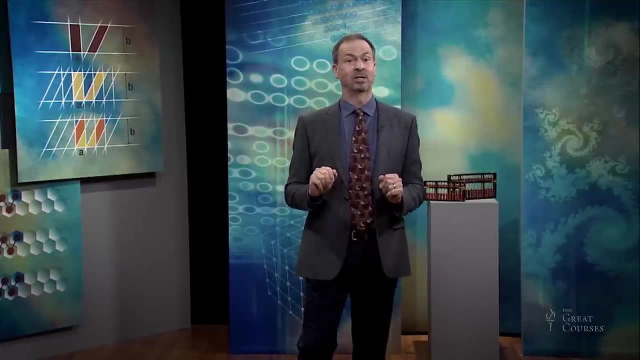 plus 3 plus 4 plus 5 is indeed 15.. Of course, as students, we wanted to know where this formula is coming from. Why is it true? Those were the burning questions in our minds, not just applying the formula to all the counting problems. 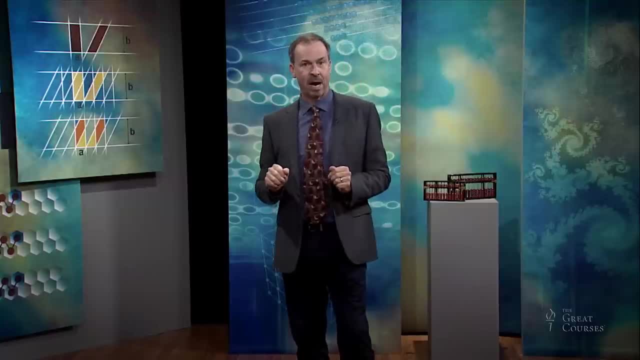 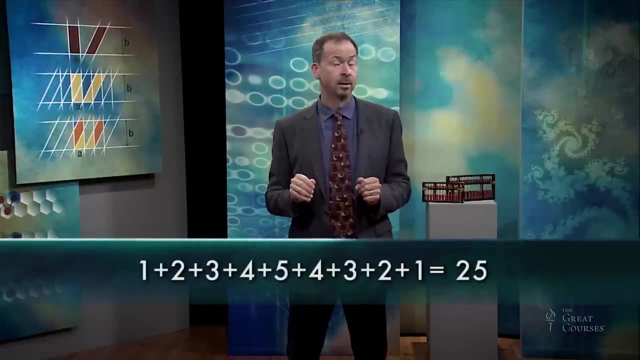 in my textbook. So how can we get this formula? Well, this test gave us something akin to this result. We have there that 1 plus 2 plus 3 plus 4 plus 5 plus 4 plus 3 plus 2. 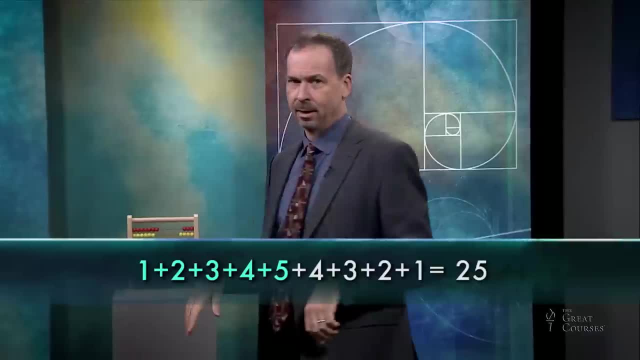 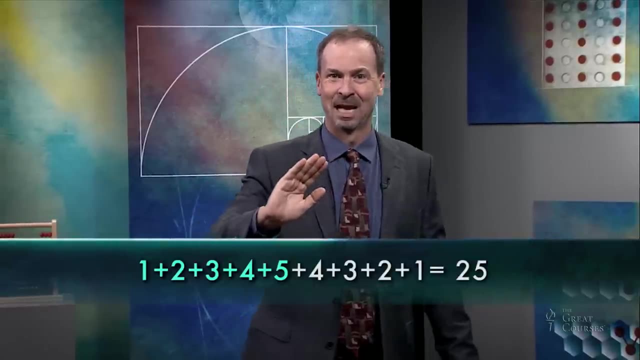 plus 1 is 25.. Can we get from this just the answer to 1 plus 2 plus 3 plus 4 plus 5?? Here's the lovely thing about doing mathematics. It's mostly about mulling and then following your nose. 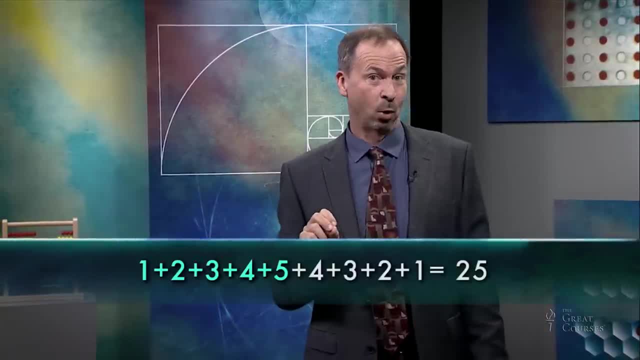 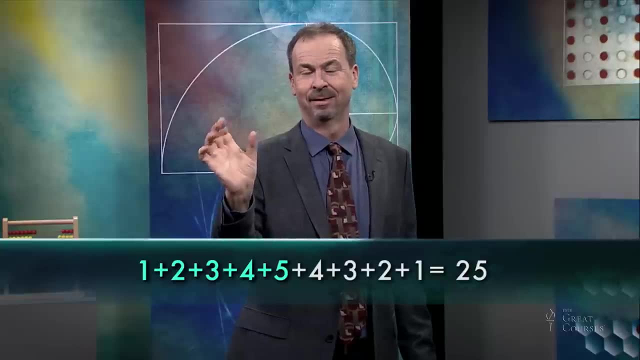 If we look at what we have, we see that the sum we want is 1 plus 2 plus 3 plus 4 plus 5.. Well, I said half. That's not quite right. The right portion of the equation is missing a 5.. 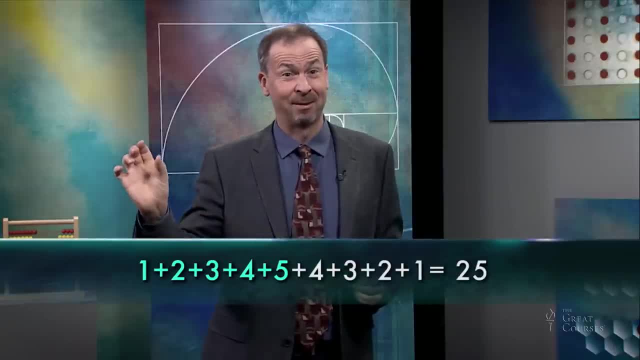 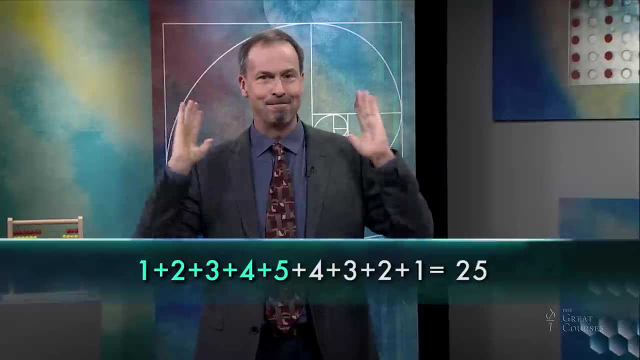 That's annoying. It's just the sum 1 plus 2 plus 3 plus 4.. Wouldn't it be lovely to see 1 plus 2 plus 3 plus 4 plus 5 on that right half there as well? Here's a piece. 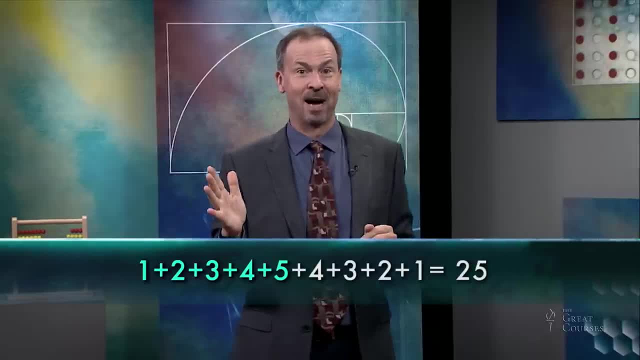 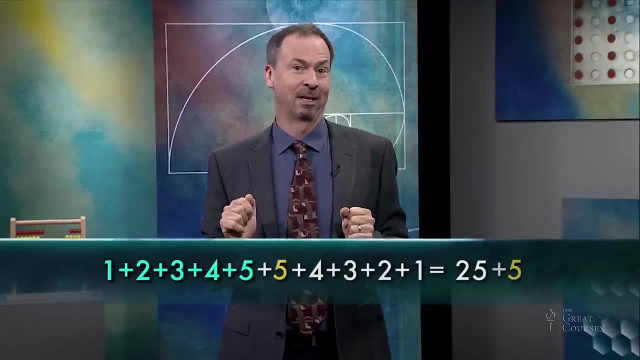 of general advice, then If there's something in life you want, just make it happen And we'll be following what's happening in the future. Let's add a 5 on the left And to keep things balanced, we need to add a 5. 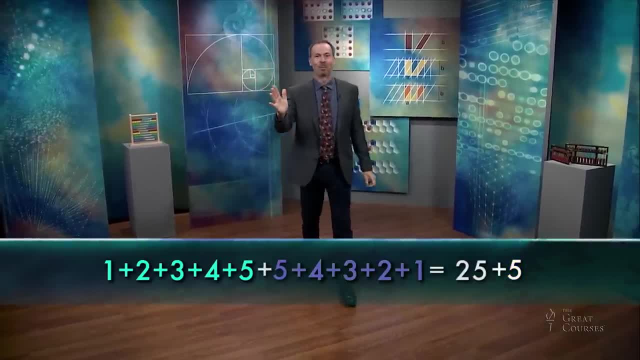 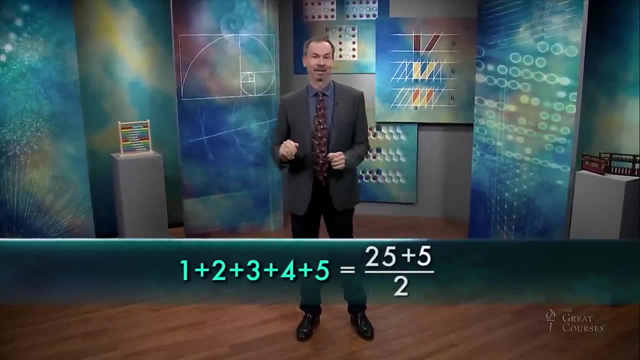 on the right as well. Lovely. Now we see two copies of what we want. Twice. the sum we seek is 25 plus 5.. So this means the sum itself is half of this: 1 plus 2 plus 3 plus 4. 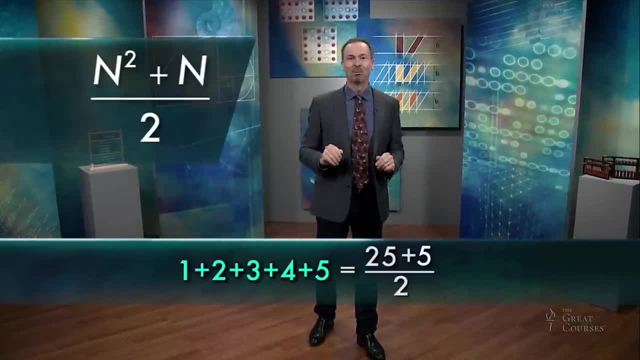 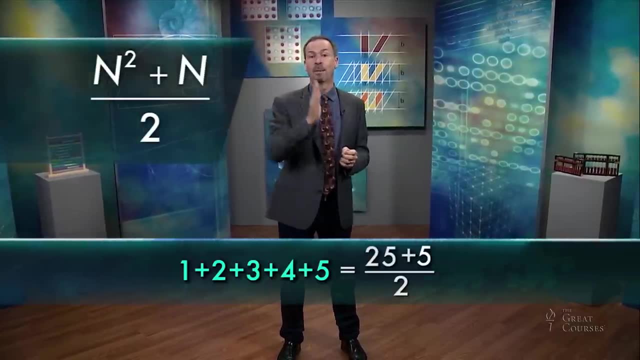 plus 5 is indeed 5 squared plus 5 divided by 2.. And this matches the general formula I had to memorize. And there's nothing special about the sum of the numbers from 1 up to n, The sum of the first. 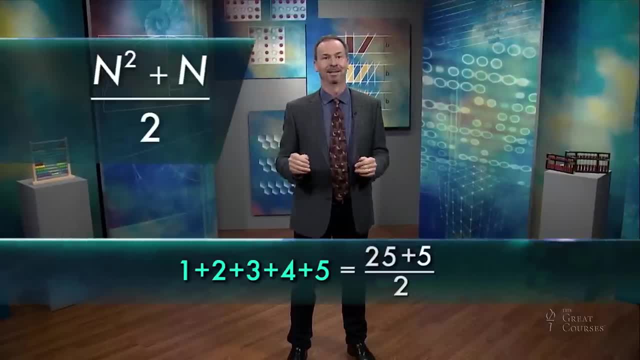 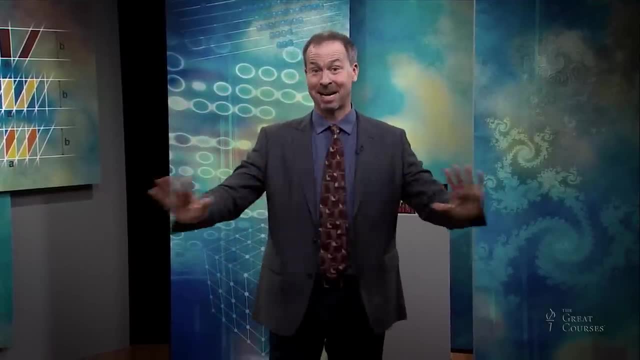 n counting numbers, that is must be half of n squared plus n. There we have it. But let's keep going. In mathematics, there really is no such thing as being done with an idea or a concept or a picture. Look at the 5. 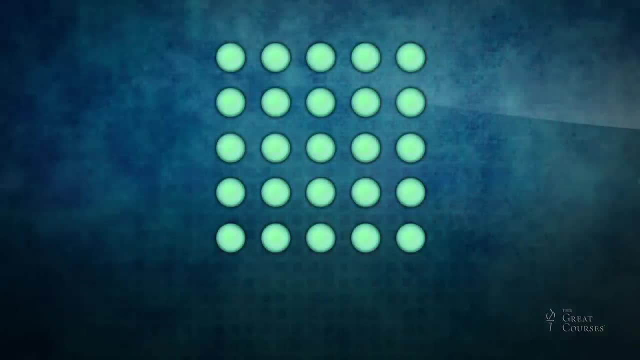 by 5. grid of dots. again This time, let me ask: do you see the sum 1 plus 3 plus 5 plus 7 plus 9 plus 8 plus 9 plus 8 plus 9 plus 8 plus 9? 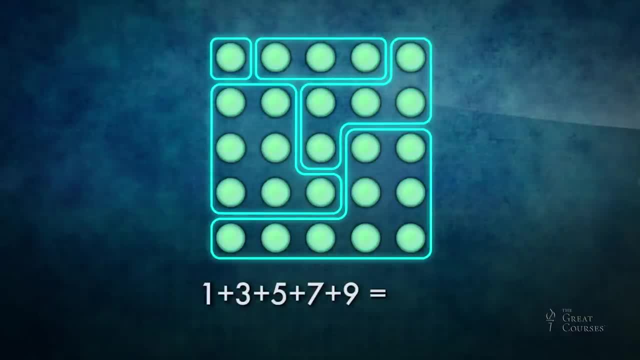 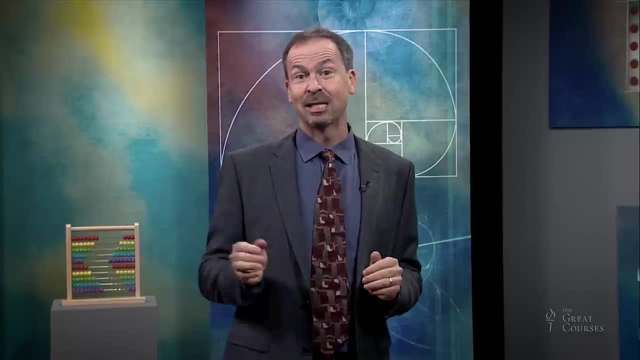 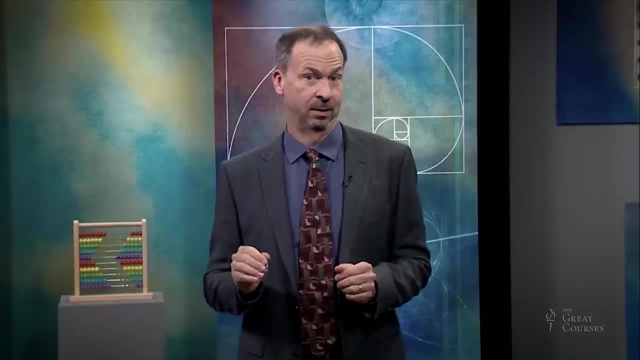 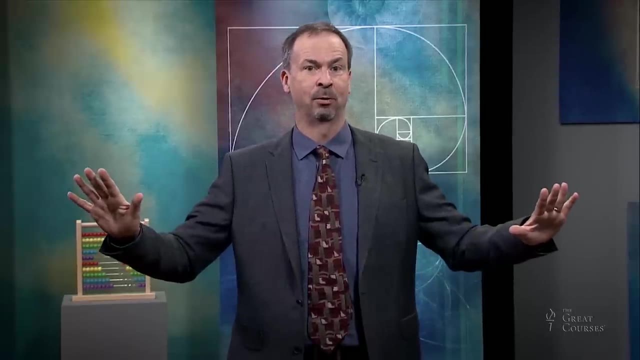 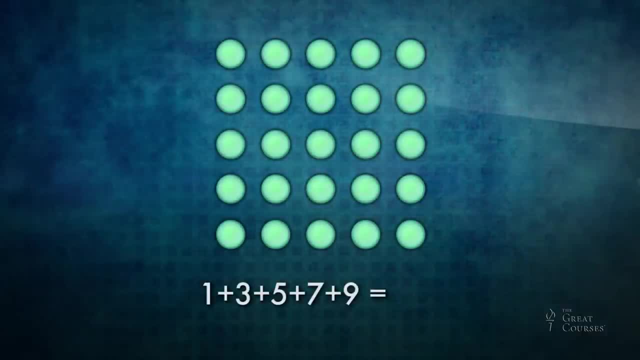 plus 20 plus 21 plus 22 plus 23 plus 24 plus 25 plus 26 plus 27 plus 28 plus 29 plus 30 plus 31 plus 32 plus 33 plus 34 plus 35 plus 36. 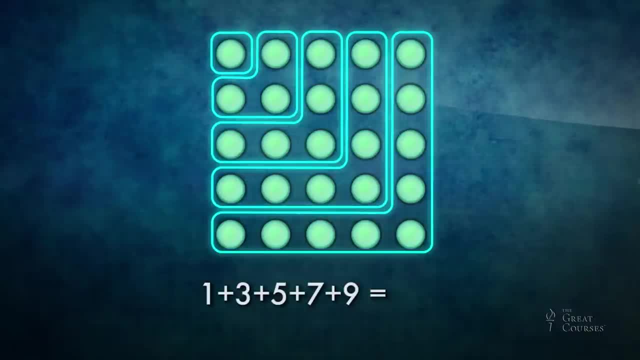 plus 37 plus 37 plus 38 plus 38 plus 39 plus 40 plus 41 plus 41 plus 42 plus 43 plus 44 plus 45 plus 46 plus 47 plus 48 plus 49 plus 50. 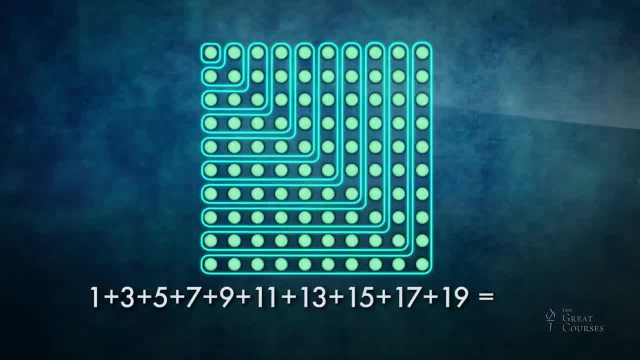 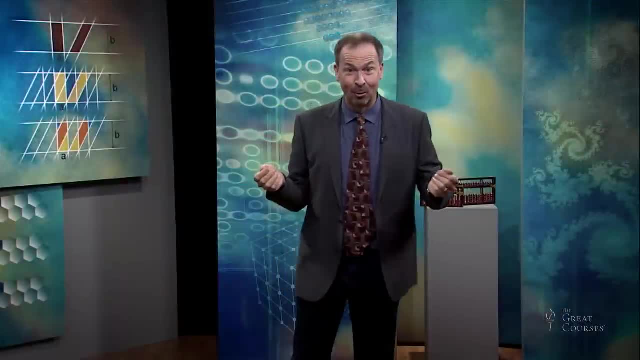 plus 51 plus 52 plus 53 plus 54 plus 55 plus 56 plus 57 plus 58 plus 59 plus 60 plus 61 plus 62 plus 63 plus 64 plus 65 plus 66 plus 67. 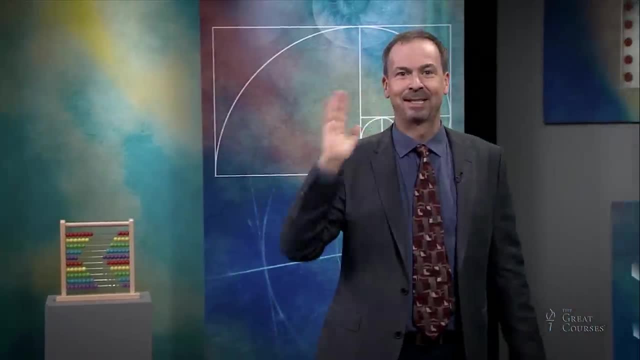 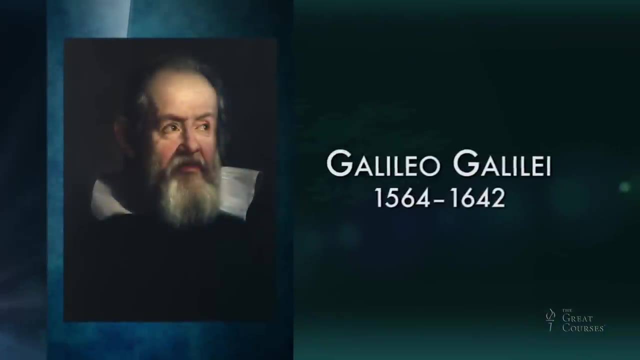 plus 68 plus 69 plus 70 plus 71 plus 72 plus 73 plus 74 plus 75 plus 76 plus 78 plus 79 plus 80 plus 91 plus 92 plus 93 plus 93 plus 94. 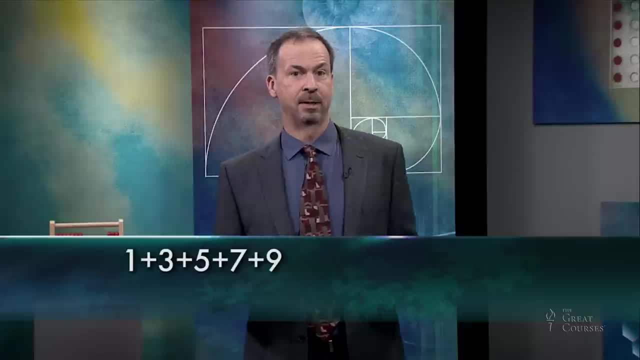 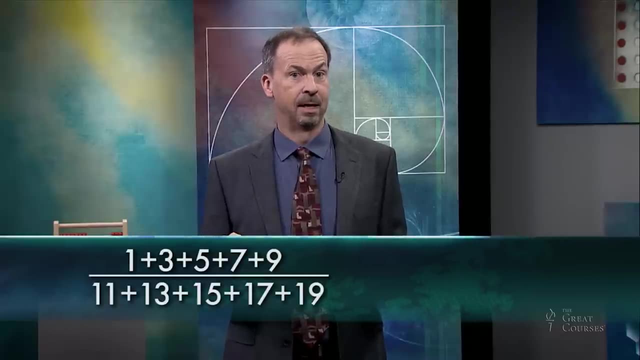 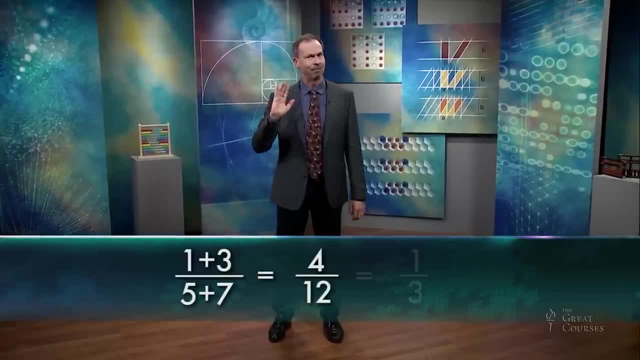 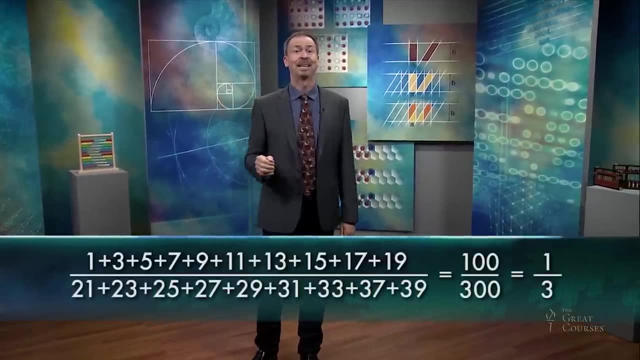 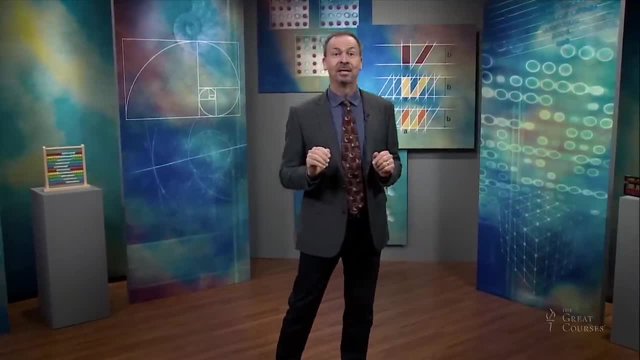 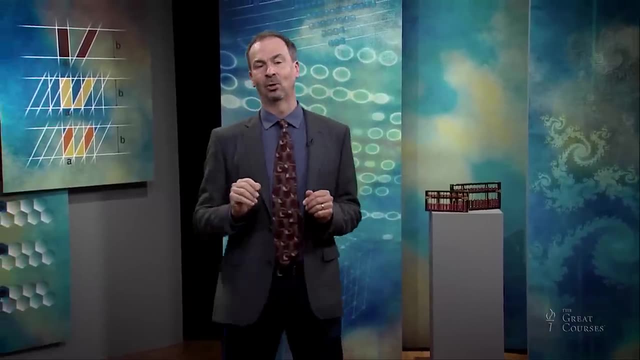 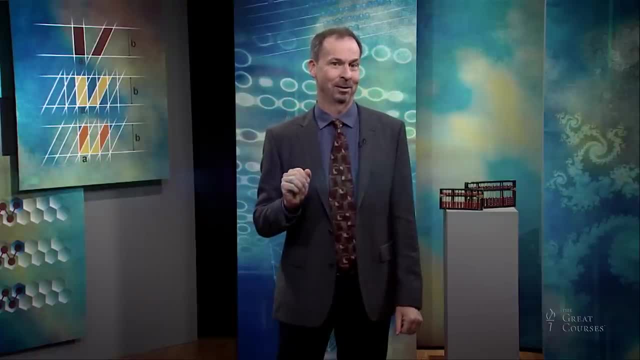 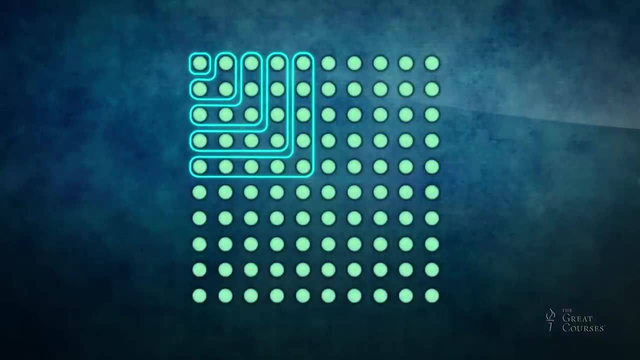 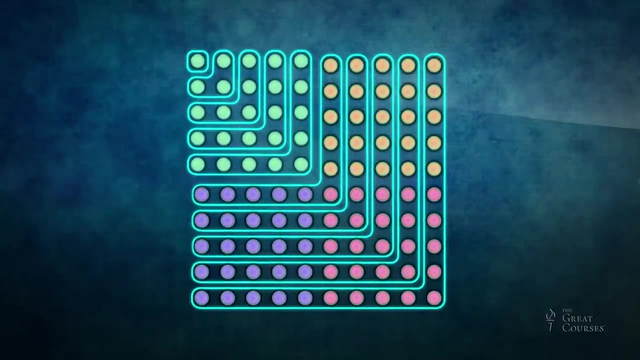 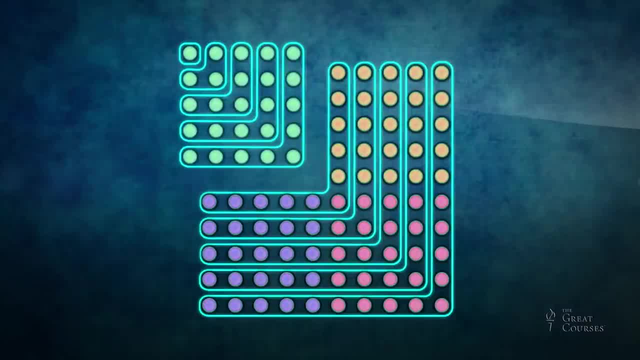 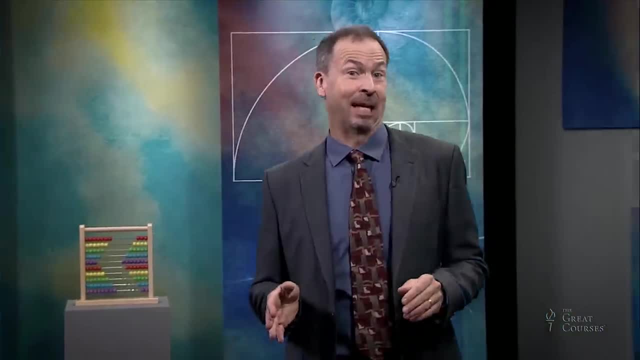 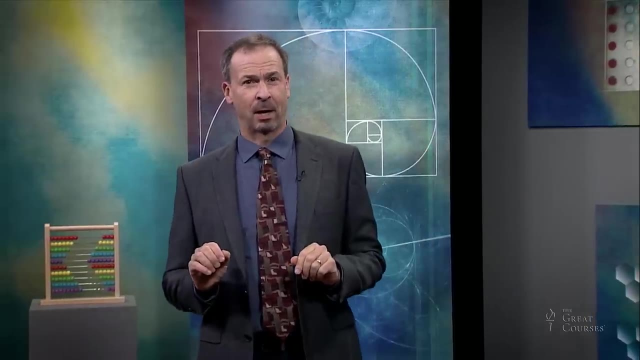 So the first five odd numbers make for one third of the next five odd numbers- Just beautiful. Next lecture we'll see how these students got negative numbers into these fraction ratios too. Amazing stuff. All right now. this focus on odd numbers is grand. 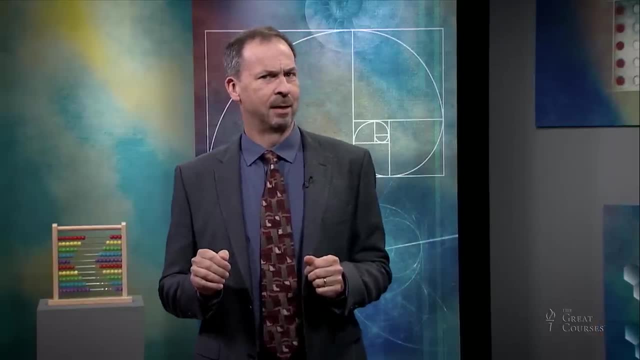 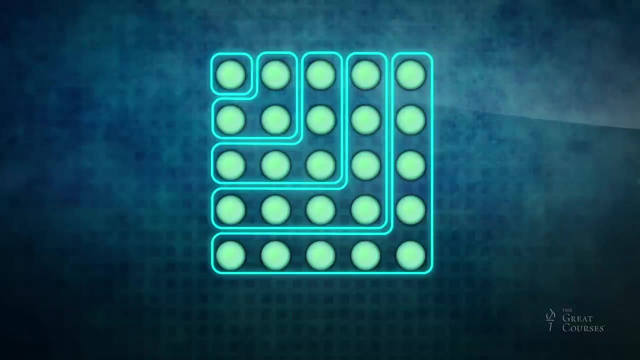 but my gut is a little perturbed by this lopsided focus on matters. Are the results about sums of even numbers as well? For example, we have a picture of the sum of the first five odd numbers. Can we get from this sum of the first five even numbers? 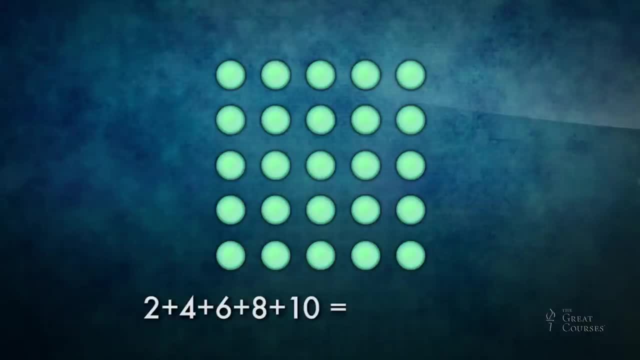 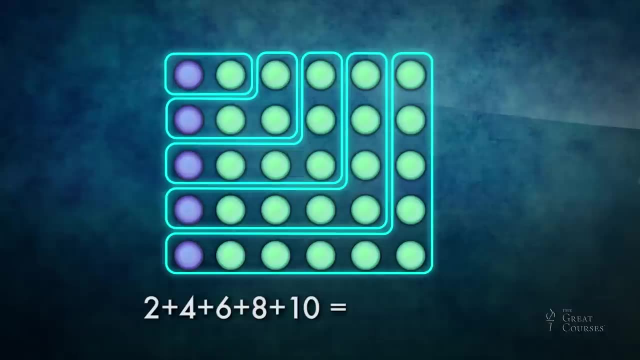 Two plus four plus six plus eight plus 10? Well, just add a dot to each L shape. Fabulous. this has turned the five by five square into a rectangle. The sum of the first five even numbers must be the five by five we had before, plus five more. 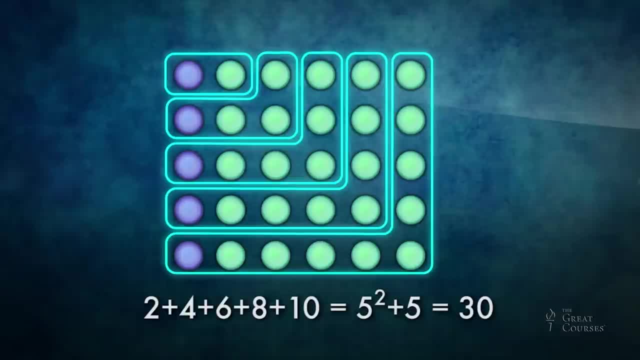 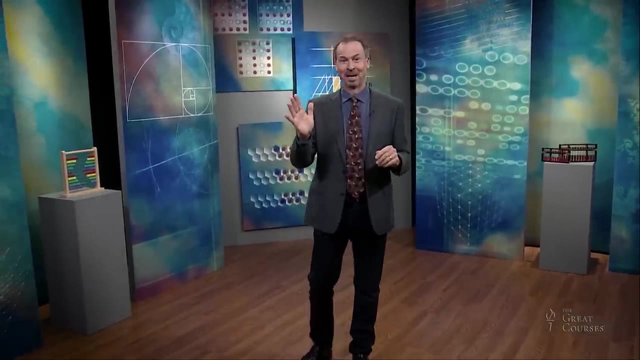 Five squared plus five, which is 30.. In general, the sum of the first five even numbers must come from the picture of N squared dots plus an extra N dots, N squared plus N. Now, as a mathematician, I'm feeling good. 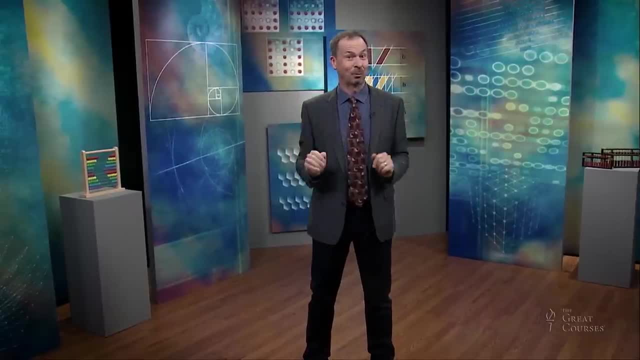 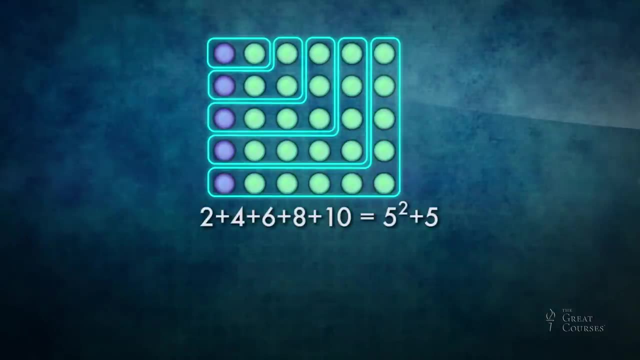 I feel we're coming full circle, as we've seen the expression N squared plus N before. Take the sum of the first five even numbers. It equals five squared plus five. Now divide everything by two. Two divided by two, four divided by two, six divided by two. 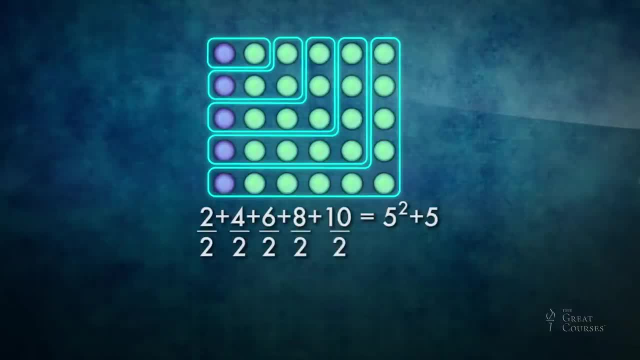 and five squared plus five. Eight and 10 each divided by two, And finally five squared plus five divided by two, And we're back to the formula: one plus two plus three, plus four plus five equals five squared plus five, all over two.